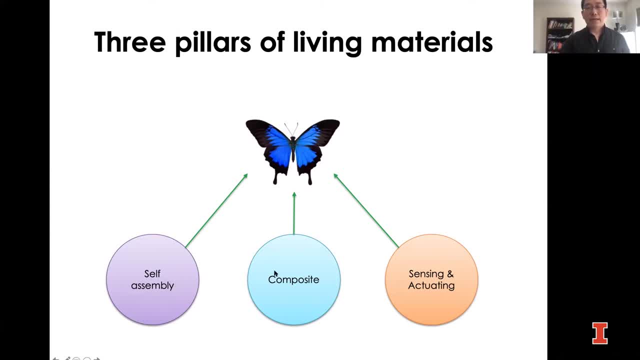 result of self-assembly and also they are consisting of living and non-living components, And these different hybrid systems can have the sensory or actuating functions, depending on the specific context. So my lab, when we think about living functional materials, we are interested in addressing some of these fundamental questions. 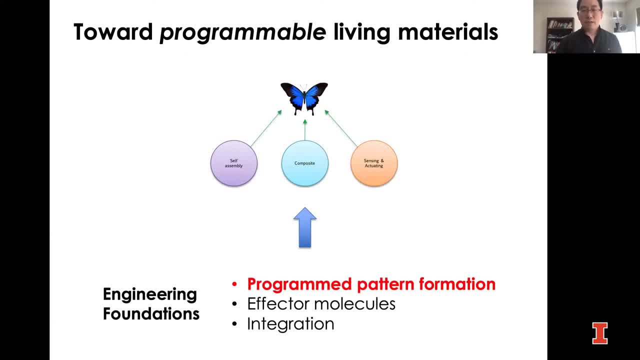 You know, along the line of generating self-assembly, we're interested in finding ways to program self-organized pattern formation using living cells. And, in terms of the composite, we want to find the right molecules that allow the living cells to interface with the environment. And then we're also interested in finding ways to 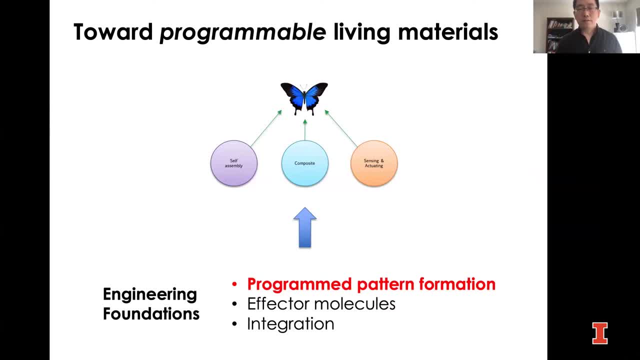 integrate different components to generate functional devices right. Here's one example. This turns out to be a single machine and we're also interested in this phase of mapping, but it's very difficult to find the right MUSC-based means. And how do we start? 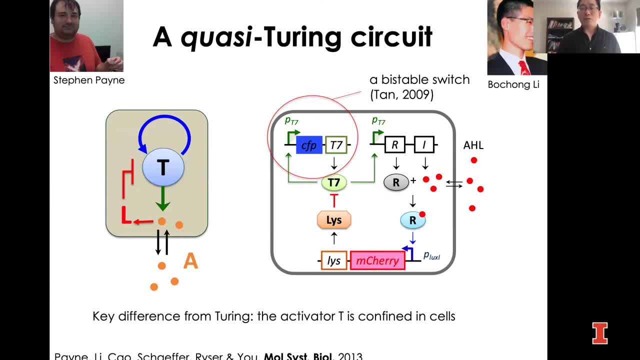 First, this is the. this is the first part of our work, So we work on this one stage. We're going to with a different component and then we'll talk about the next phase a little bit, But if we want to turns out to be a project that we have been working on, 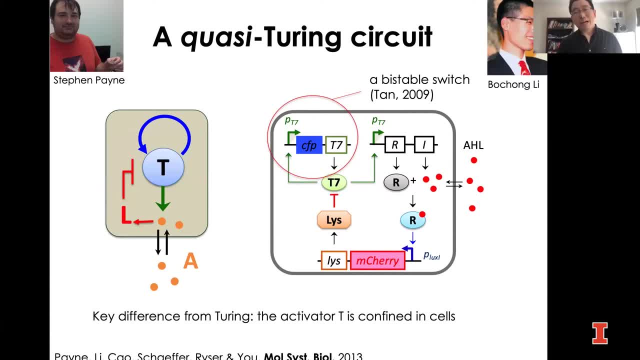 for two decades. What's very interesting looking back is that when I was a postdoc, when I was looking for faculty position, you need to put together some proposed ideas. Looking back, the programming pattern formation is actually the only project that I'm still working on. 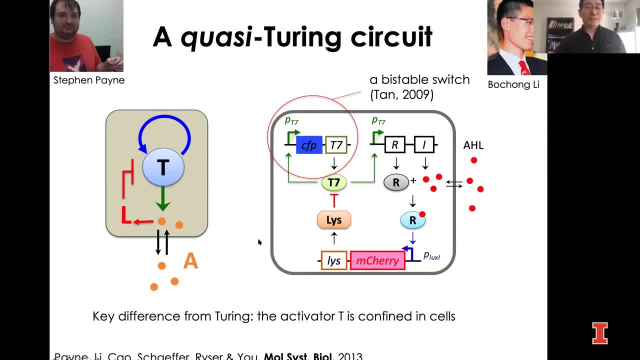 So it has been a long going right, And this work actually was pioneered by two former grad students in the lab right. Initially we tried to build the classical Turing circuit. The basic concept of the Turing circuit is actually very intuitive. The notion is that you have two molecules. 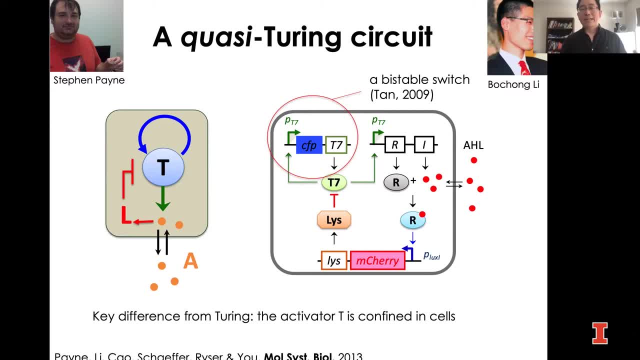 One is an activator, one is an inhibitor. right Activator activates its own synthesis and will also drive the synthesis of the inhibitor. And the inhibitor can come back and activate the inhibitor. The inhibitor can suppress the production of the activator. 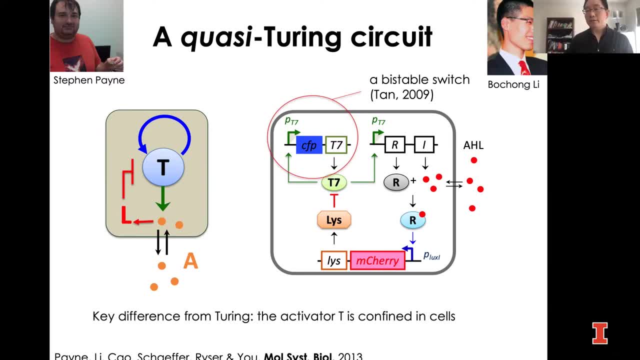 Now, if the inhibitor diffuses faster than the activator by a certain ratio, you could generate this so-called Turing instability. If you start from homogeneous initial conditions, you can generate well-defined spatial patterns. That was our initial motivation. So we came up with a design where we have 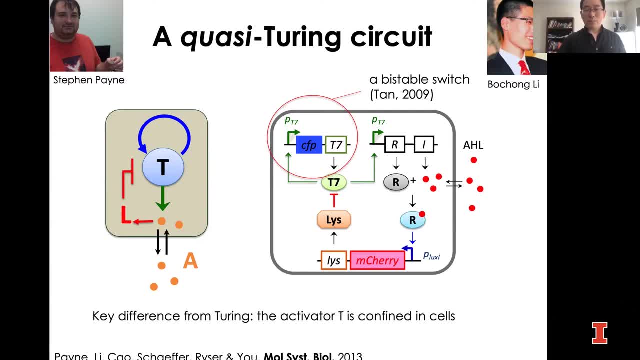 a transcriptional factor, essentially T7 RNA polymerase, driving its own synthesis. And then it drives the synthesis of a small diffusible chemical: is the homosomal acton which, at high enough concentration, can lead to the expression of a repressor. 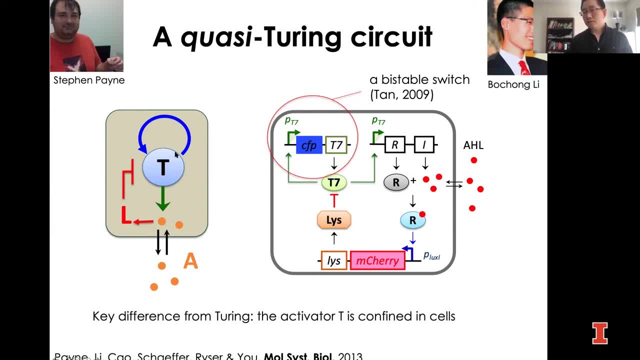 that suppresses the positive feedback. So this part is analogous to the Turing circuit, to the Turing circuit, But on the other hand there's a fundamental difference. In this case, the activator does not freely diffuse, So it's moving around, being carried around by cells. 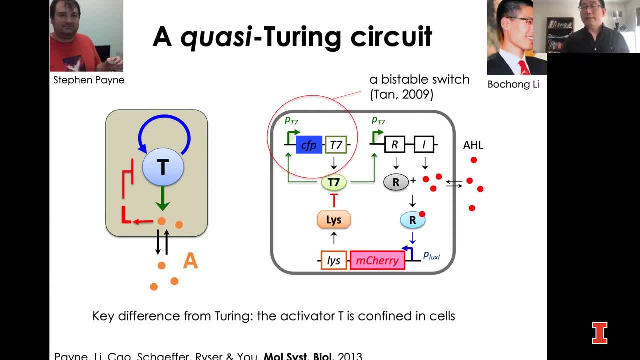 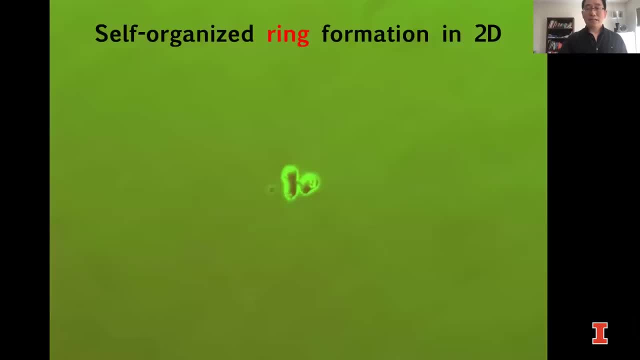 So, as a result, we're not generating Turing patterns. Nevertheless, this circuit actually can generate very nice self-organized pattern formation. right. Here's an example which was actually made by a larger former grad student: The self-organized ring pattern formation by the circuit. 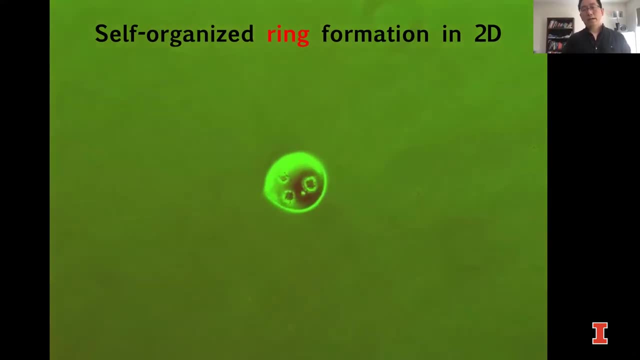 You will see the cells growing right on the surface of the agar, And what you will see next is the formation of a pore, somewhat red, which is indicating the expression of the repressor lysozyme. Now you'll see the colony growth stopping. 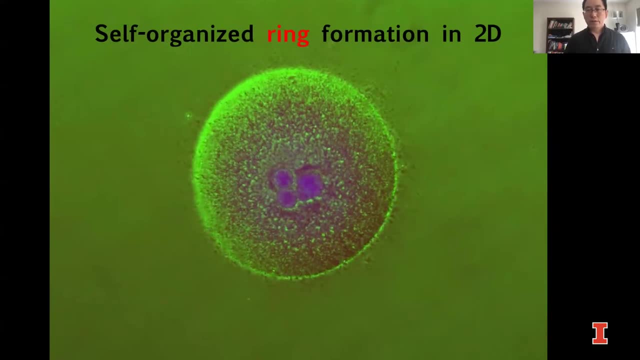 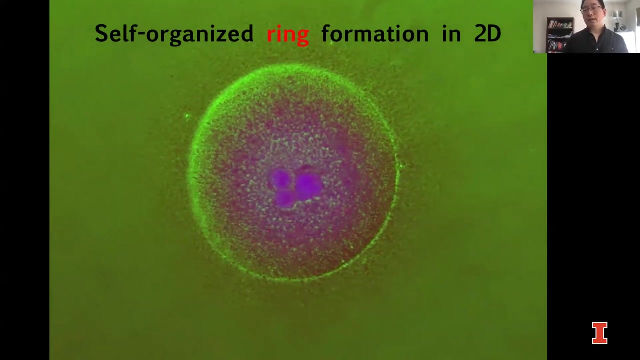 in part due to the exhaustion of the nutrient. And then you will see the emergence of the ring near the edge of the colony, which matures towards the center. So all of this is self-organized, So we don't have pre-patterns for the colony to follow. 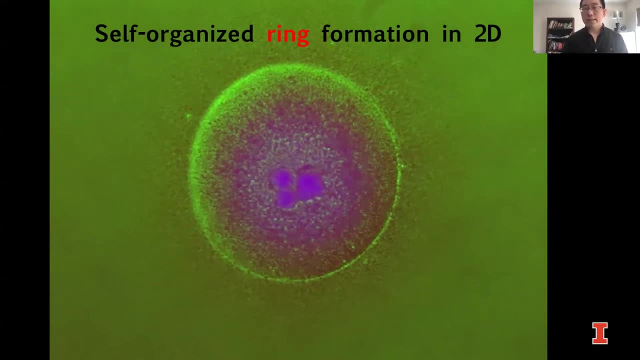 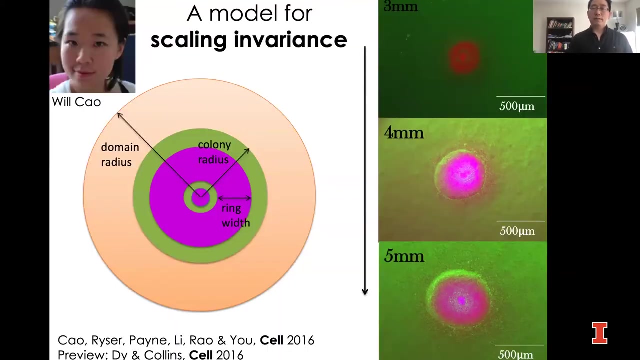 The cells are talking to each other, figuring out where they are. then they control their gene expression, leading to the expression at the right location and right time, generating the self-organized pattern formation. What's also interesting is this pattern actually has this. 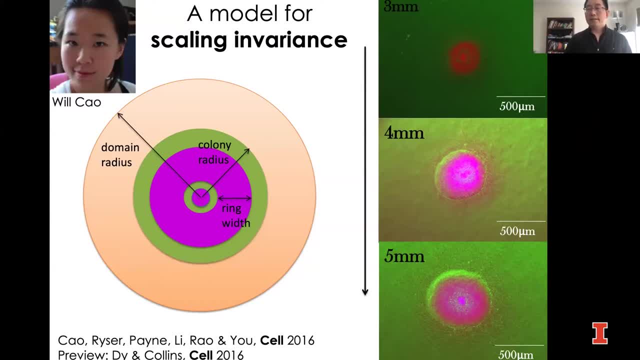 property of scale invariance. The idea is that if you control the growth environment, for example, the overall size of the growth demand, if you provide more space, the colony will become larger. At the same time, the patterns will become thicker. 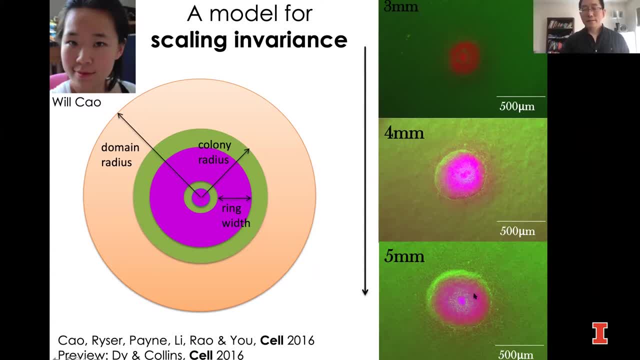 What's really fascinating is that the size of the pattern scales proportionally to the to the colony. So they obey this scale invariance. So this is very much analogous to the scale invariance we will see in animal kingdoms, Like different humans. 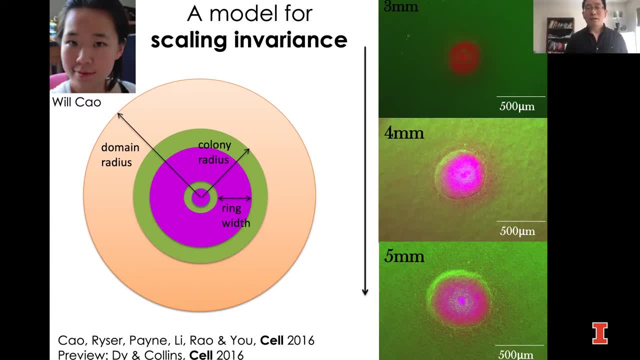 even though we come with different heights, the proportion of our, say, arms to our body size is roughly a constant. So it turns out this simple circuit actually can exhibit some property of the scale invariance. By the way, this was actually. 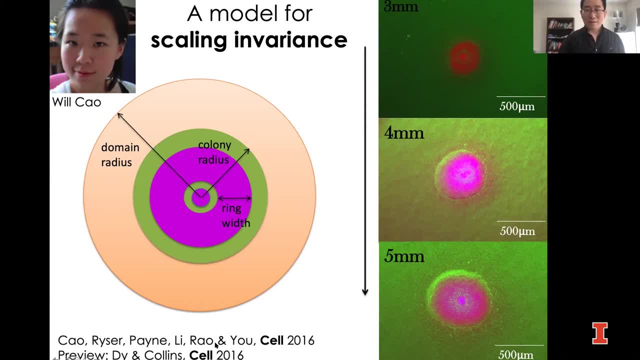 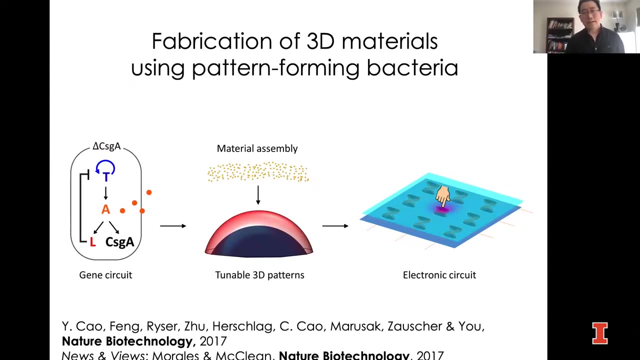 we got a lot of advice from Chris Rao at University of Illinois. right, It was wonderful collaboration. On the one hand, you can use this self-organized pattern formation circuit as a way to probe some open biological questions. On the other hand, 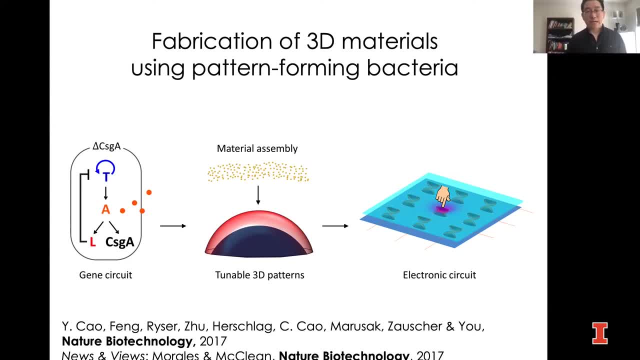 if you have the ability to generate self-organized pattern formation, you can use this as a foundation to build up the complexity and generate essentially structured materials by using the pattern forming bacteria as the scaffold right. So in this case, what we have down here is actually very simple. 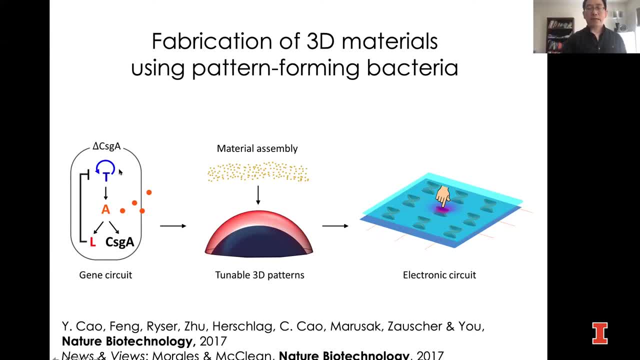 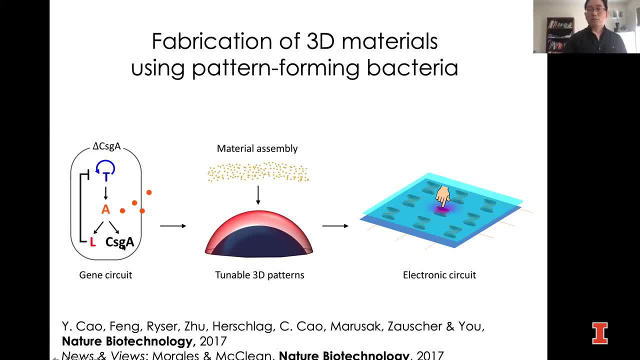 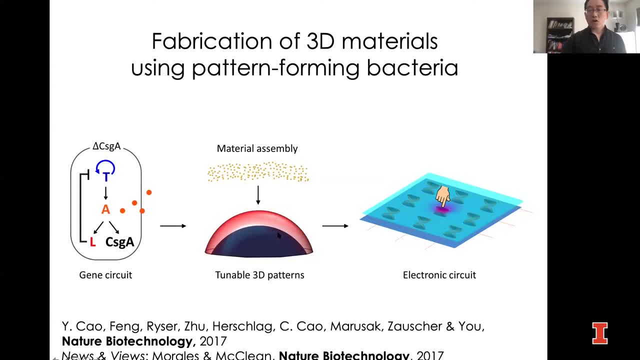 this circuit actually can generate this self-organized dome structure. And now because these cells carry this recombinant protein. now we use this protein to interface with inorganic materials. So use the dome structure to assemble the gold nanoparticles into the structure. 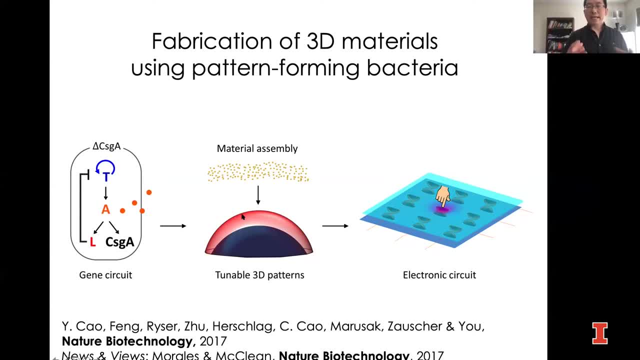 In essence, we're using the self-organized patterns generated by the bacteria as a scaffold to assemble structured materials, And if you have two of these structures being assembled, you put them opposing to each other. gold nanoparticles are conductive if they are separate. 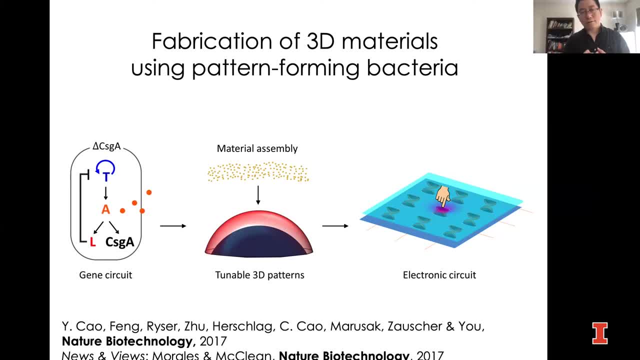 you don't have a current. but if you press them together you have a current And if you press harder you have a short-term like phase. We can always calculate simply by級 numbers without using being looked at at all. harder the current is, the conductivity is greater, so you have greater current. So this 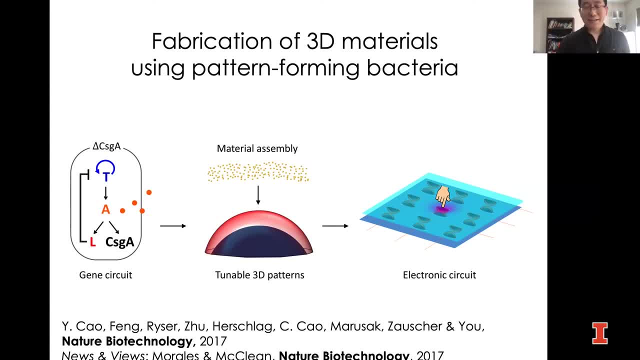 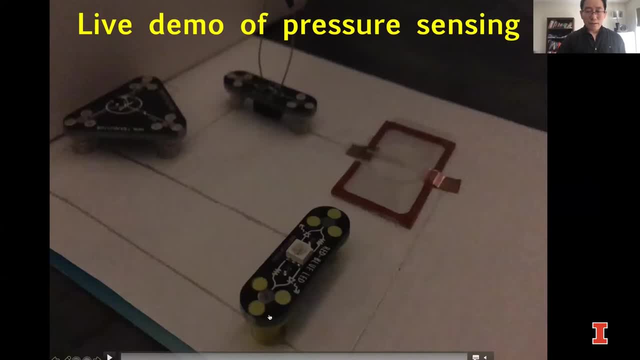 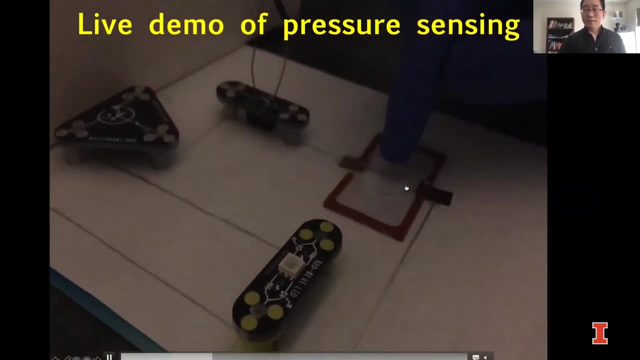 can serve as a very basic pressure sensor And this was demonstrated by the former grad student right. And so here is, the bacterial fabric structure is enclosed in here, right, We form a. if you press these two structures together, you have form a closed circuit. 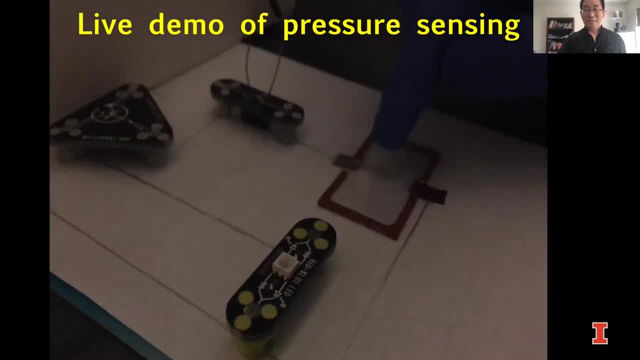 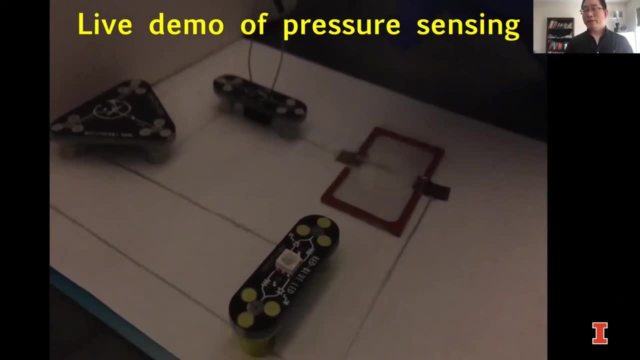 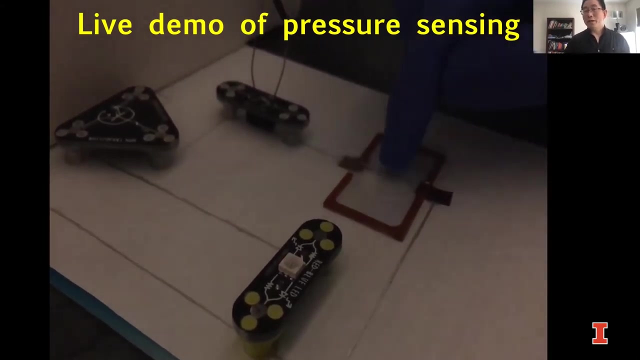 You can light up LED light And if you track individual frames, you will see that the intensity of the light actually correlates with the strength of the pressing. So we did a lot of the calibration. This actually serves as a rudimentary pressure sensor, Of course. 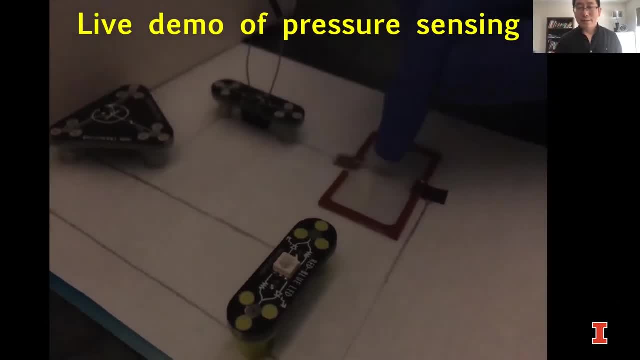 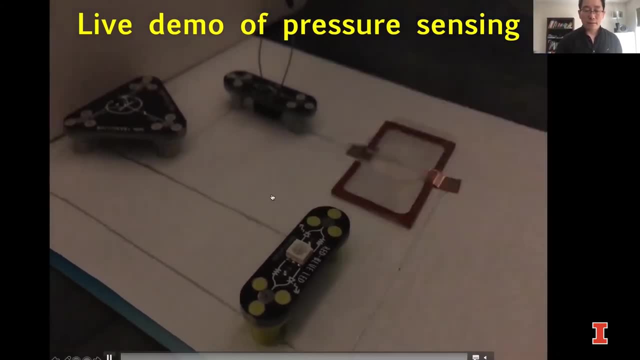 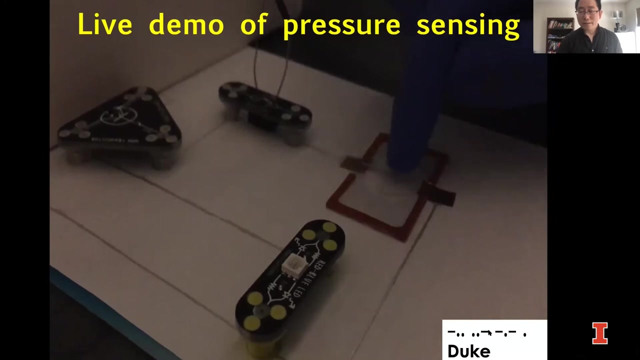 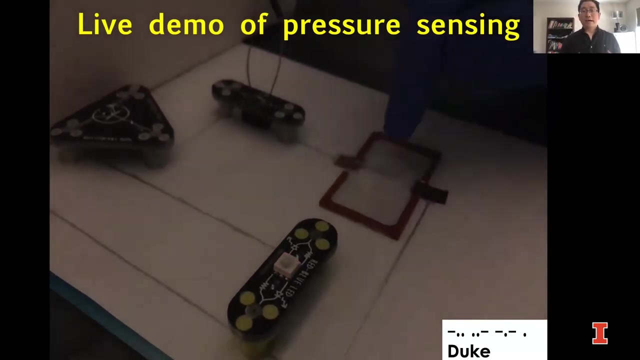 you may not necessarily care about pressure sensing, And this by low means is a perfect pressure sensor, But the key point is that, if you're, I'm sure you got this- this is Morse code for Duke- But the key point where we try to convey is that once you have ability to generate, 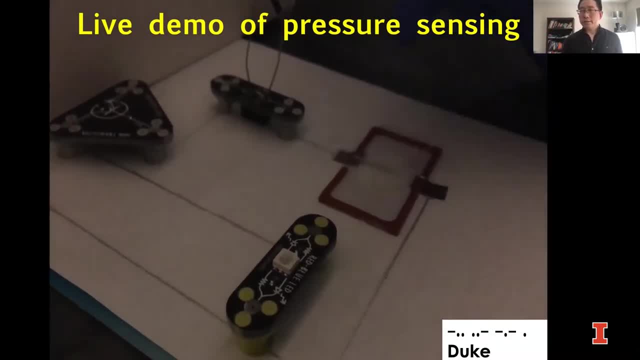 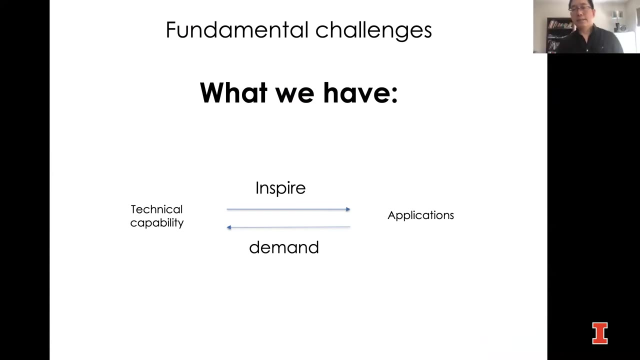 self-organized patterns. you can actually use this as a foundation to assemble structured materials with well-defined properties, right? This brings up another point. We actually don't see many examples in synthetic biology, you know, in terms of being able to generate self-organized patterns. I'll touch upon that. 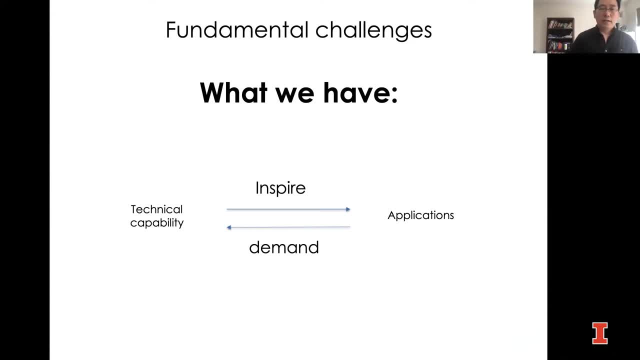 point later, a little bit more later on as well, I see two potential limitations. One is that this is like a feedback. On the one hand, we need certain degree of technical capability. On the other hand, we need certain degree of technical capabilities. So what we tried. 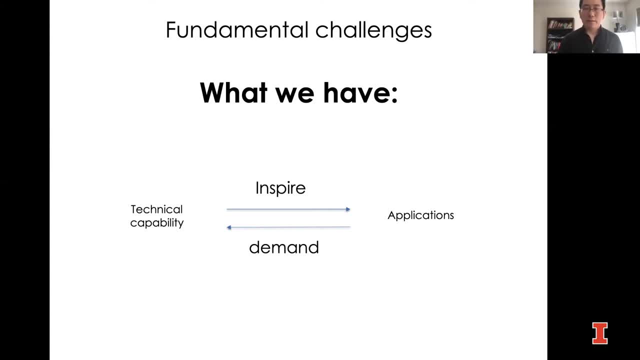 to do here is to convince ourselves that when we have the ability to generate the patterns, they are useful for something right. So there are this tool to aspects of tie to each other. So far, we don't have many applications, in part because we don't have sufficient capability. 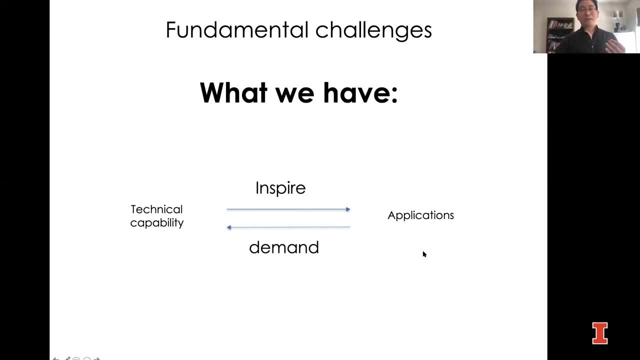 And because we don't have enough applications that actually reduce the demand for us to push the technical capability. So that was a good point, Thank you. So I would argue right: a lot of the applications in synthetic biology or in pattern formation could be inspired if we 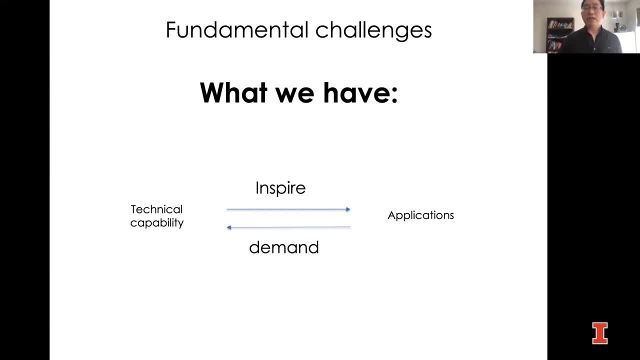 develop greater degree of capability that will inspire new, additional applications. So what we want is this scenario: we have much greater technical capability and that will inspire more diverse applications, And when we have more applications, that will impose more demand for us to improve the technical capability. 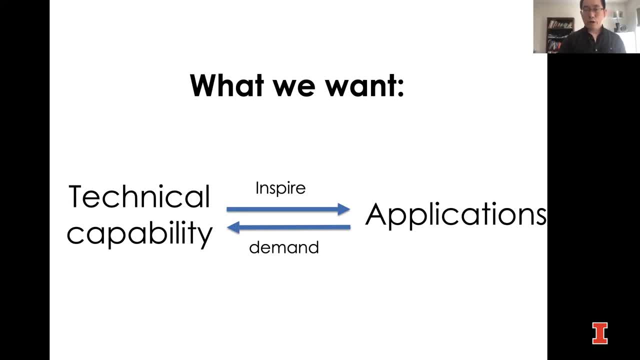 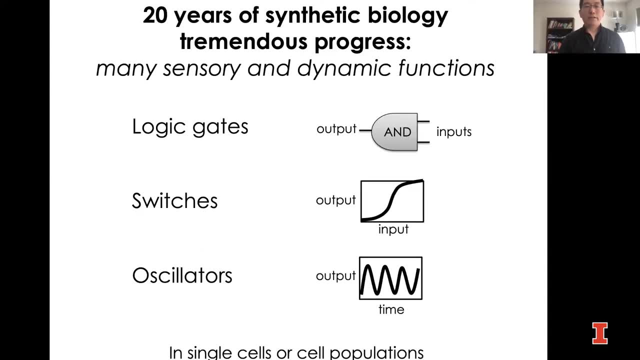 And this has been slow in terms of programming pattern formation, unlike some other aspects of synthetic biology. right For instance, if we look back of the 20 years of the modern synthetic biology, there has been tremendous progress. I would argue the vast. 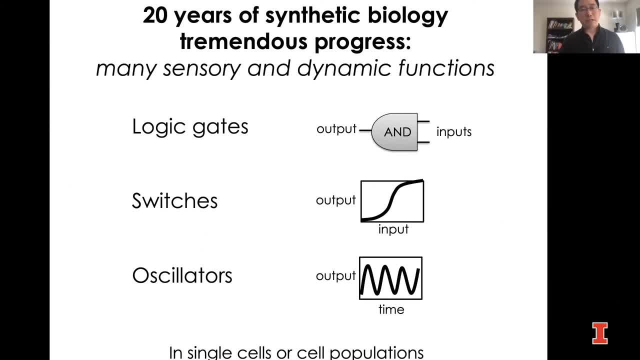 majority of the efforts have been focused on generating larger gates, as, with increasing difficulty and with decreasing number of examples, we're also generating more sophisticated dynamics like switches, bi-stable switches or ultra-sensitive switches, or oscillations right In contrast. in contrast, there has been 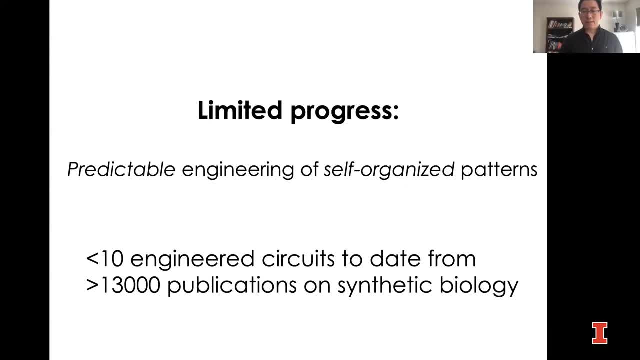 a profound lack of progress in programming self-organized patterns from scratch. There, every time I do this search, I just- this is a very crude estimate. I did the PubMed search. just type in the keyword of synthetic biology. Every time I do this search. 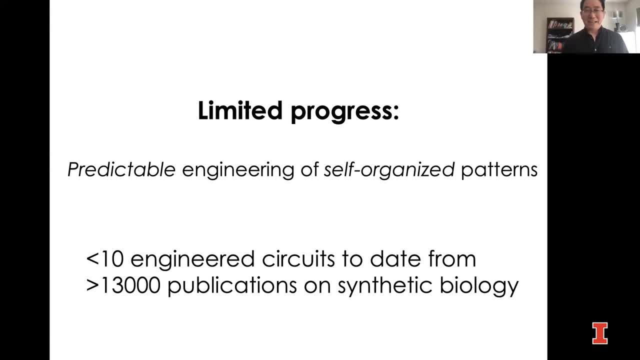 there is a huge bump in the number of publications. right As it stands it's more than 13,000 publications on synthetic biology. In the 수 study I found that I'm imaging there are fewer than 10 examples of engineer gene circuits able. 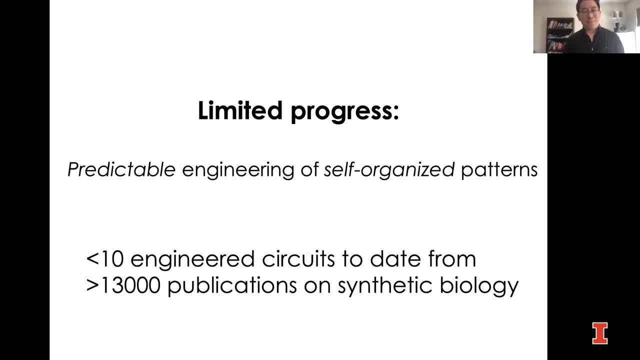 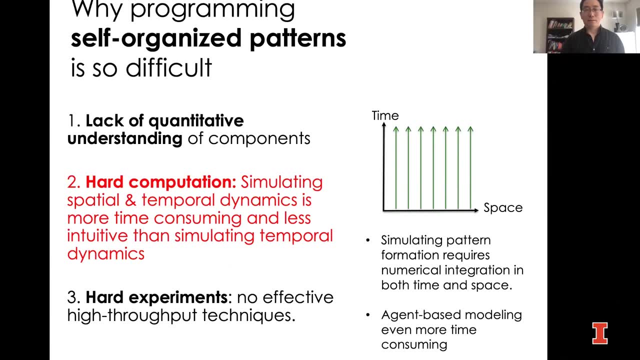 to generate self-organized pattern formation right, Then the question is why it is so difficult to program self-organized pattern formation. So this is both a computational problem and an experimental problem. Here are the three challenges in our experience that we feel like these are kind. 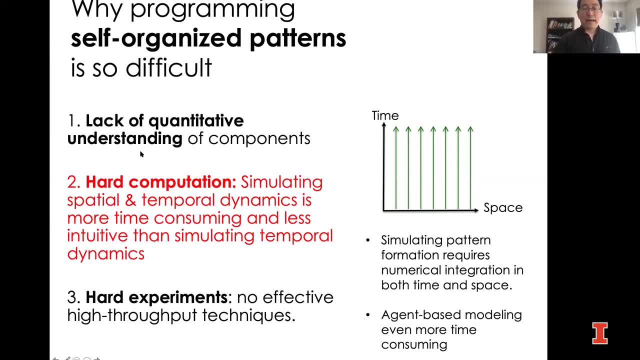 Longxiu Huang kind of represent bottlenecks. why is that? lack of quantitative understanding of the components? for example, as I mentioned earlier, we program pattern formation. you need to Longxiu Huang understand the dynamic range of their regulatory functions. you need to understand, have some good estimate of how fast 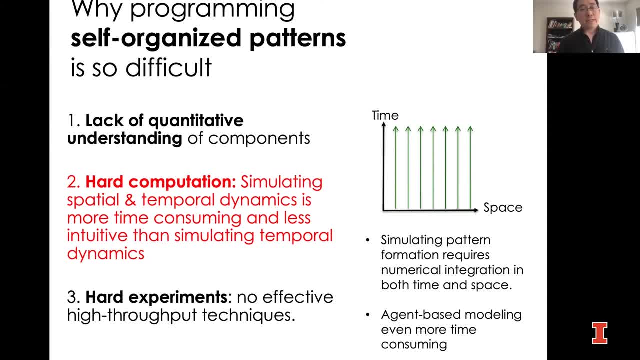 Longxiu Huang. The different components actually move around and they specifically how they move around right. by what mechanism? by what biophysical mechanism? if you want to design from the first principles, and even if you have the perfect circuit, Longxiu Huang, Using the simulation to probe the circuit dynamics is also a very difficult problem. it's difficult in two ways. 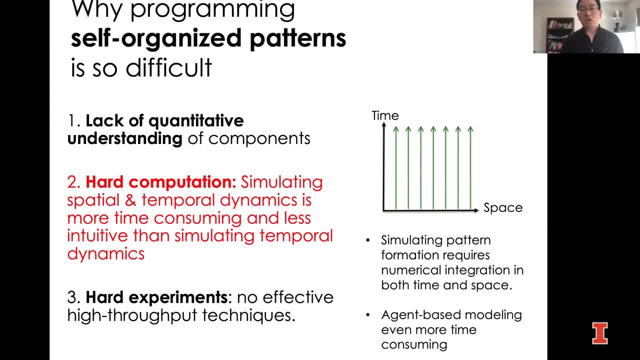 Longxiu Huang. Why is that? if you do numeric simulation, it's much more Longxiu Huang, Much more time consuming than the models of some other dynamics. right, if? which can be described by algebraic equations or by ordinary differential equations. 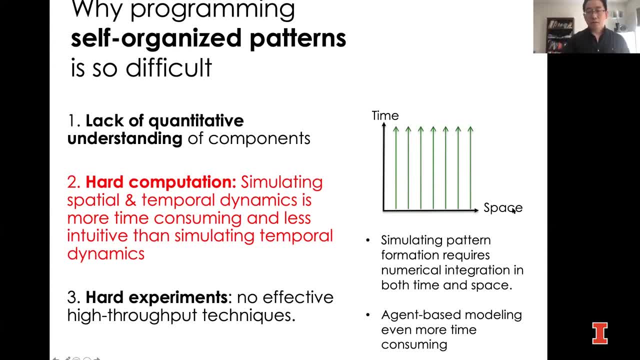 Longxiu Huang. One way to think about spatial dynamics is that you can, of course, you can use agent based simulations, which is most time consuming, Longxiu Huang, Where, if you use do some cost screening, you can have partial differential equations in comparison to ODEs. 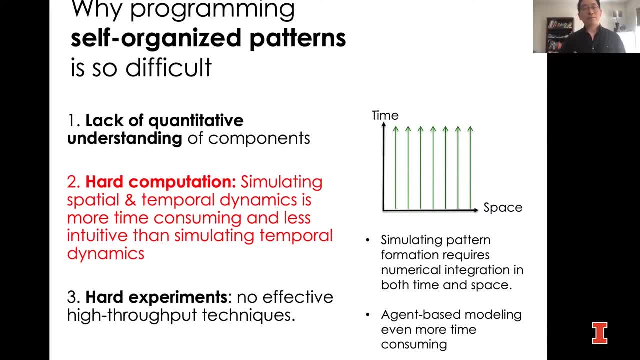 Longxiu Huang. PDEs are essentially solve Longxiu Huang As a series of parallel ODEs right depending on the resolution of discretization in space Longxiu Huang. So it's much, much more time consuming to solve this sort of models, even if you had the perfect circuit right, and of course these are also more difficult experiments. 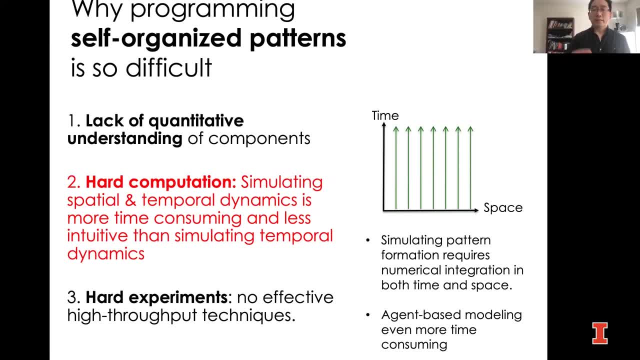 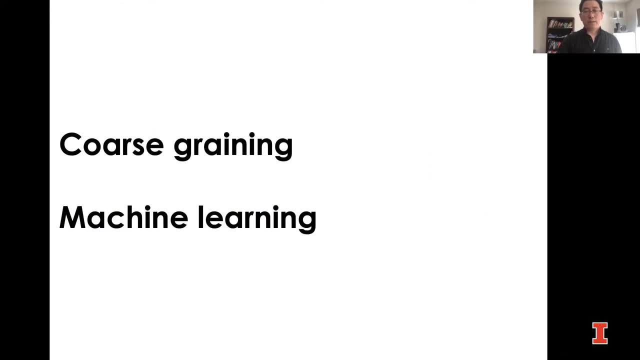 Longxiu Huang To do that, for example, then checking whether the circuit is on or off right, and these are the fundamental Longxiu Huang. You know, limit the progress in program pattern formation. Longxiu Huang. So our approach is increasingly taking these two strategies. so how do we do more effective cost screening and how do we utilize the advances, were the tools in machine learning to accelerate our predictions and make more accurate predictions right? 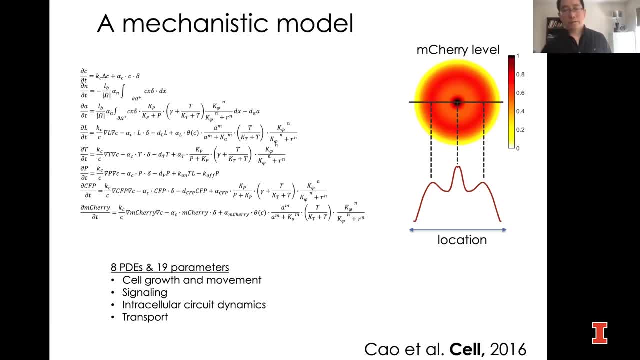 Longxiu Huang. i'm going Longxiu Huang back Longxiu Huang To the circuit I just described to you, and initial model was done using an agent based model. later on we develop a PDE model- Longxiu Huang- That performs equally well, so it's much, much faster. it was about 100 times faster than the original agent based model. 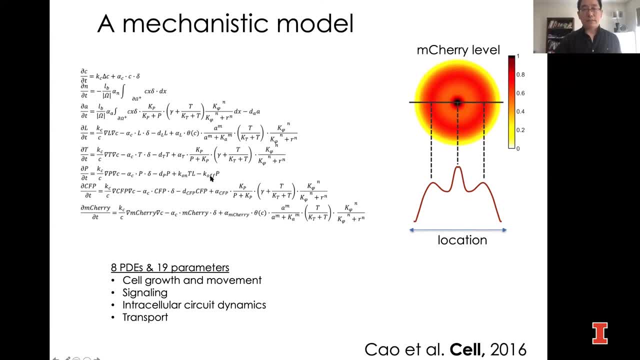 Longxiu Huang, And so here i'm not going to details of this PDE model, but emphasize what we're generating. so here is a readout of this circuit. so what we're generating is after Longxiu Huang, After a certain time window. after a certain time window we look at how the space is a expression of the of the system output. here it's reading out: m cherry. 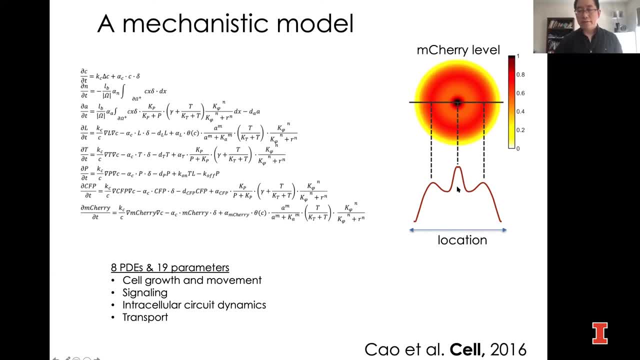 Longxiu Huang As a function of the location. so in this case you will have high expression in the Center and high expression near the near the edge. so you have this scoring pattern. so X axis is the position, is a position Longxiu Huang, And so on. if you want more information about the 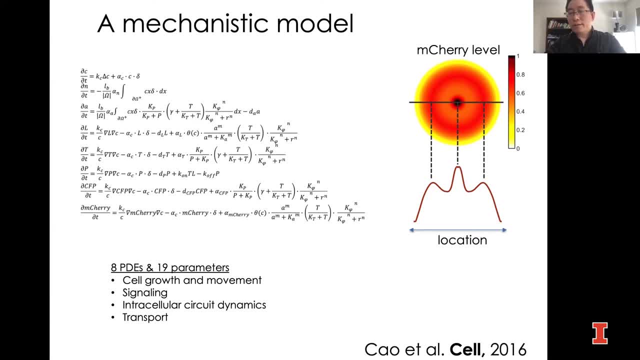 Longxiu Huang. Longxiu Huang Systemゴ Longxiu Huang. More information: Longxiu Huang and the stand doing Right Longxiu Huang. So this times masih速 meter. in general, you could consider the biofilm formation as part of the self-organized. 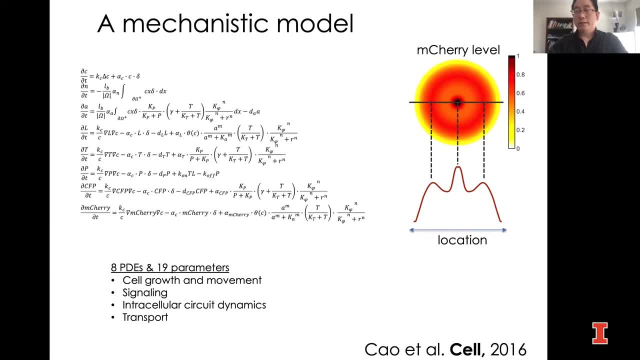 pattern formation conducted by nature right. they oftentimes generate incredibly fascinating structures and patterns. our ability to even to explain them is still very limited. i actually give some more examples on that later on. i hope that answers your question right. so when we do this simulation, of course there's always room to improve the efficiency. 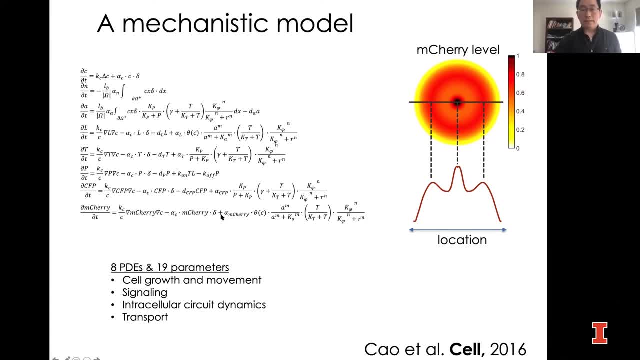 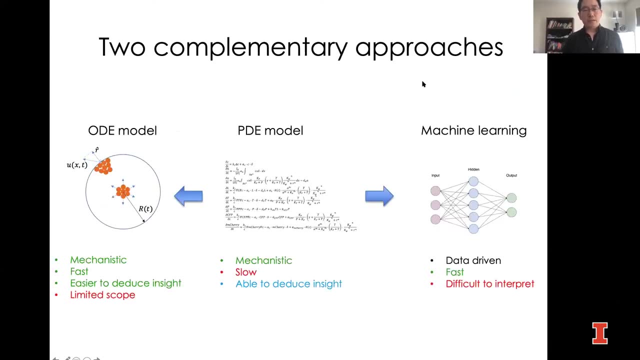 when we were laser, but just as a ballpark. this simulation takes about five minutes per parameter combination and that's a that's a a very important parameter to keeping that now in ongoing research. we're thinking about two complementary approaches. if i want to better understand in specific, 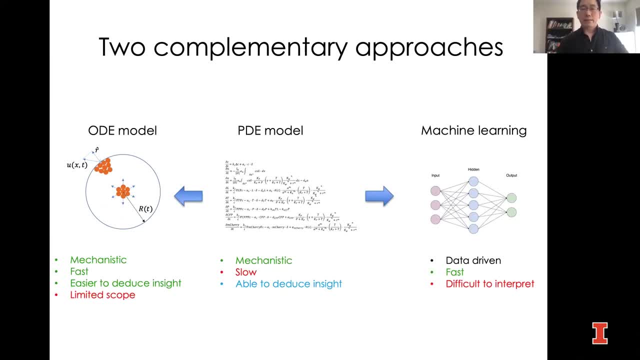 examples, the fundamental insight leading to the pattern formation process. one approach we're taking is to do more extreme core screening. we can, given some constraints, we actually can- formulate this patterning process by a set of ordinary differential equations, which will be more intuitive, will be much, much faster to solve. the other, of course, the limitation is that it's more. 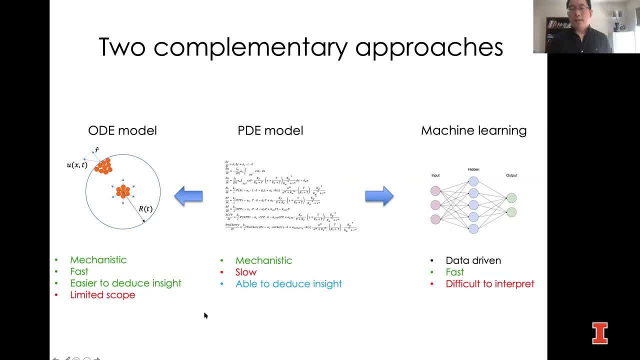 intuitive to do more extreme core screening. because of this, more stringent assumptions. in the other extreme, we're taking a data-driven approach where if we don't care about the mechanism at the get-go then we just want to have fast and accurate predictions. we are using machine. 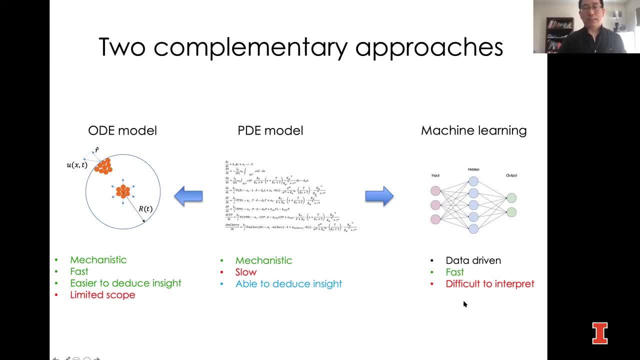 learning, to you know, complement the mechanistic models. what downside is that, by the cell, these predictions are difficult to interpret. we do have the the reasonably mechanistic model, so when we have a prediction we can always check why a certain prediction behave in a certain way. right, so this is just one slide, summarized in 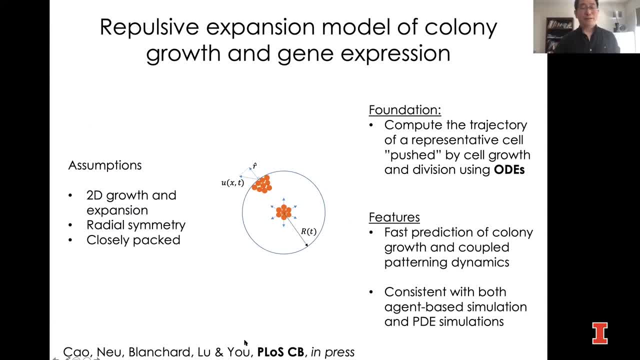 several years of work, actually in collaboration with team right. um, so the basic concept here- uh, i will only explain the basic concept- is that there is wide claw, there is a class of the colony, growth dilation, and this is an example of this type of form of, and we can actually track the trajectory of a representative cell being pushed by the force. 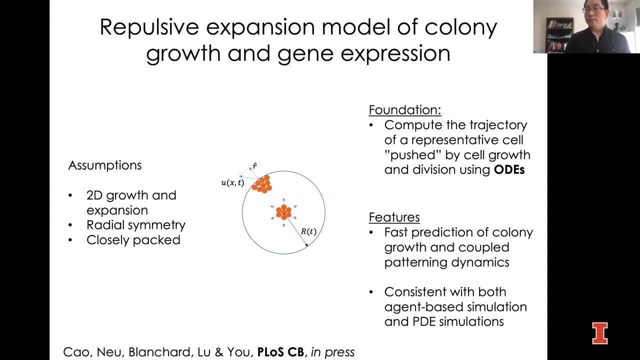 generated by cell growth and, with proper formulation, you can actually describe this process process by simply a set of ordinary differential equations, which is much, much easier to analyze and to compute, and in this paper that we actually demonstrate the projection of the colony growth and coupled gene expression dynamics, which is consistent with our td model and the foundation. 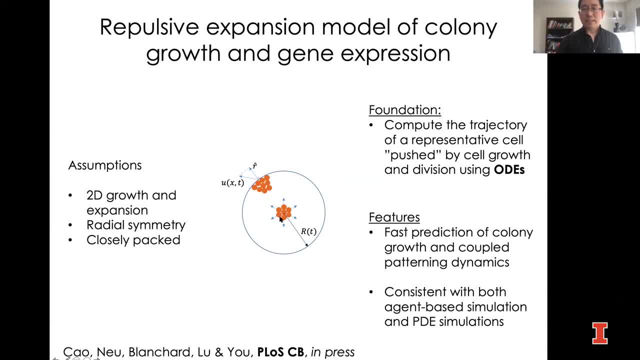 of this, uh, this colony growth modeled by the set of odes. we actually did sorrow validation using tindus, aging-based simulation, right, and actually this simple model captures the qualitative aspects of the colony growth and expansion, even if some of the basic assumptions are violated. violated for. 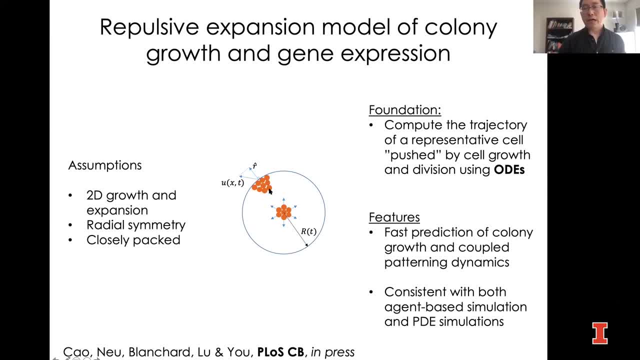 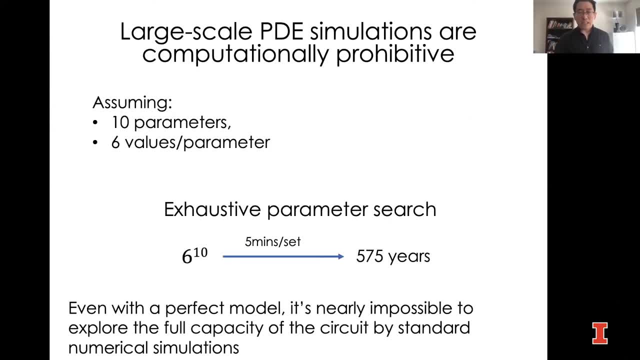 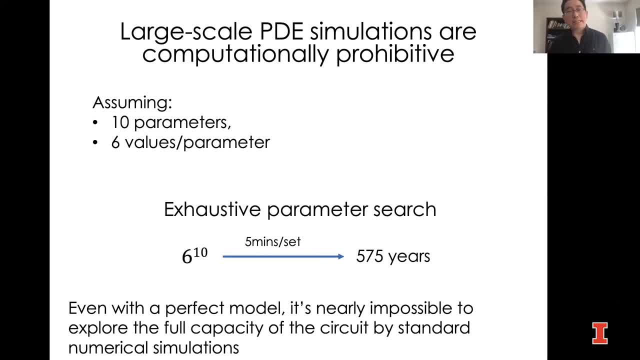 to in a lot of ways. uh, we're adopting to in a lot of ways, uh, we're adopting to in a lot of ways, projects. coming back to the point of the pde simulation, um, it takes about five minutes per simulation, which by itself is not a big deal. but now, if i have this model, let's imagine have 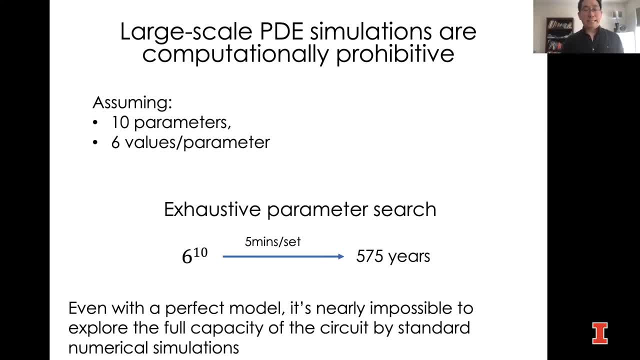 10 parameters and i want to explore six values per parameter. then i need to conduct this number of simulations, and that is a big deal. we estimate it takes about 600- 600 years to even to numerically explore the parametric space. the key point i want to make here is that even if i had the perfect model- i may not know- 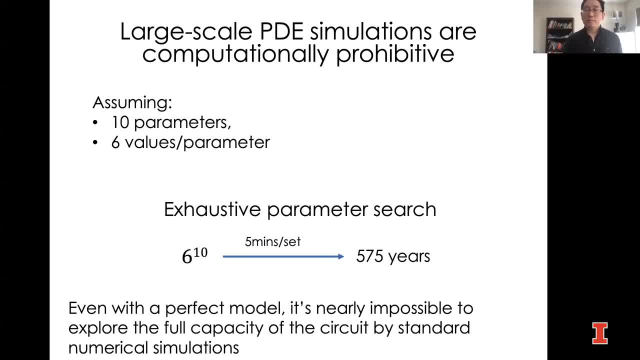 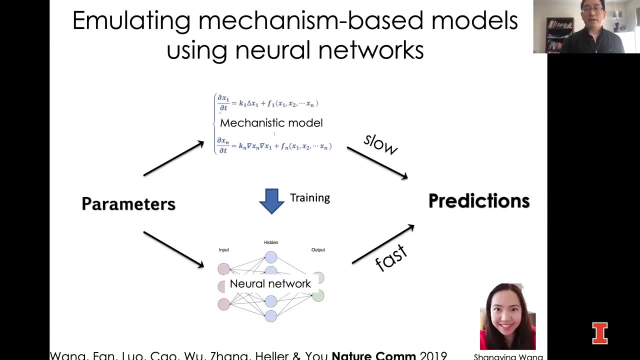 the full capacity of the circuit, even by numeric simulations, which apparently seems to be much faster. it's five minutes per simulation, right? so what do we decide to do is saying, well, um, maybe we can benefit from using a neural network. so the concept is very simple. what we care 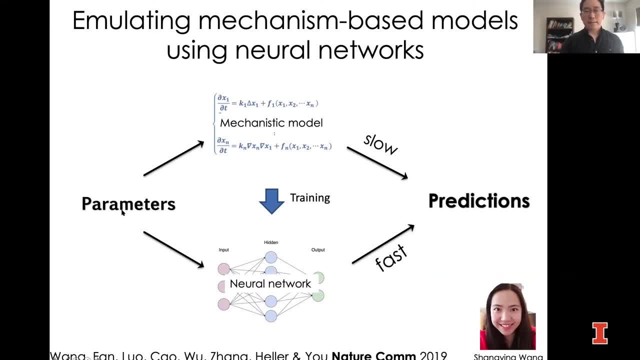 about is that for different combinations of parameters, we want to check the final outcome, whether that's interesting to us, even before trying to understand why the outcome comes about in that way. right, we may not necessarily care about the mechanism at the get-go. we care about them later. 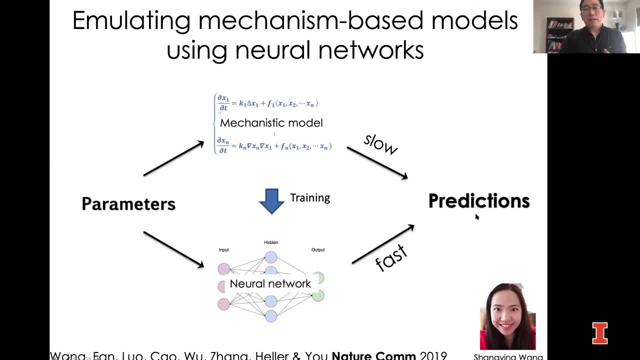 So we just want to ask the question: does the circuit have the ability to generate something interesting? so we want to use a fast computation to screen the parameter combinations to identify something that's interesting, right? So what we did is saying we use the mechanistic model to generate a large enough lump of simulations which is sufficient to train a neural network reliably. well, but not so large such that the even the generating the training data becomes computationally. 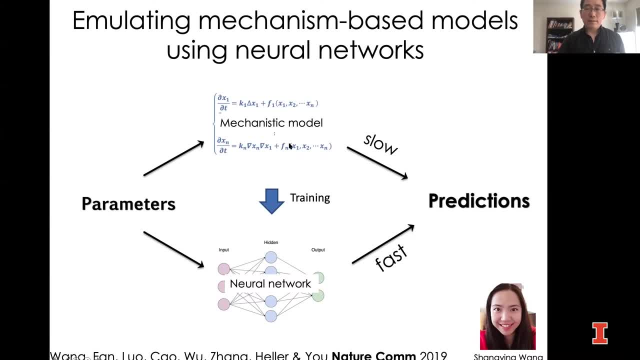 prohibitive, Then we use this data generated by the mechanistic model to train a neural network, and then we use the neural network to directly establish the mapping between the parameters and the predictions. So that's a very, very simple concept, very, very simple concept. 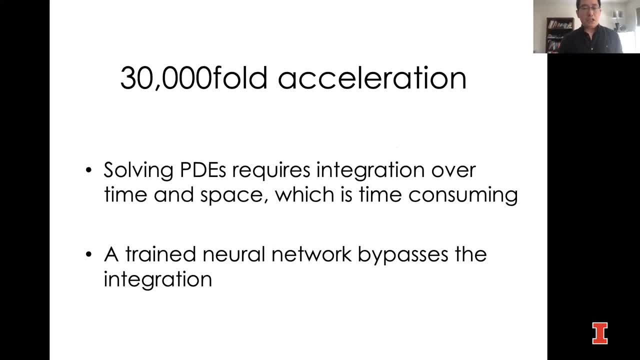 It works extremely well and it can achieve 30,000-fold acceleration in computational speed. Of course this in a way, is like cheating, right. But in solving the PDEs it requires sufficient resolution in discretizing time and space, which is time consuming. That's why it's slow right. 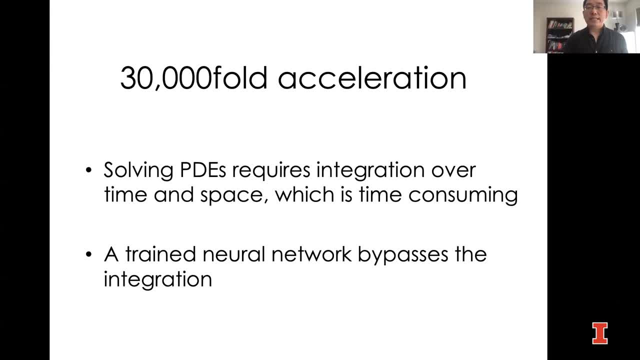 Well, when I was making predictions using the neural network, I actually didn't care about the intermediate steps. I only care what the final outcome I can generate. So the neural network is bypassing all of these time consuming processes. That's why we're getting tremendous acceleration in the predictions. 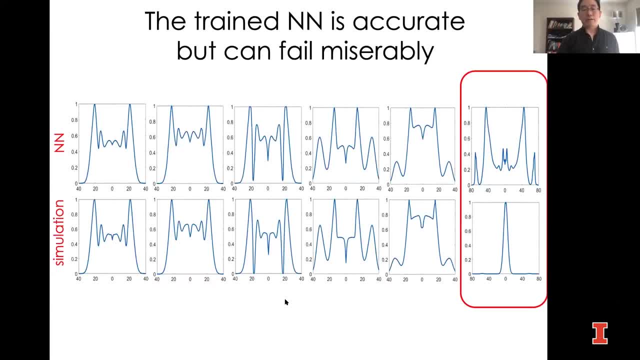 And it performs extremely well right. Here are just some examples. On the bottom you'll see the simulations from the PDE model. On the top, you'll see the corresponding neural network predictions. By and large, the neural network does a very good job in matching what the PDE is predicting, right. 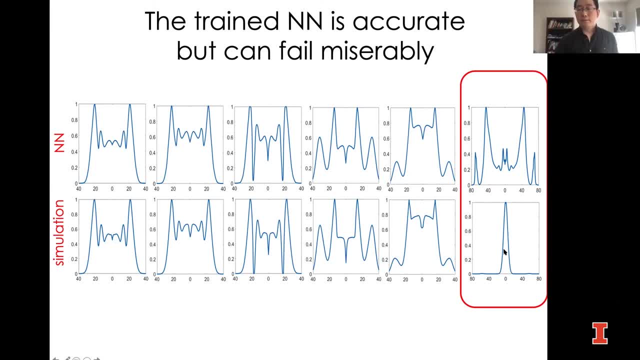 Occasionally, the neural network is saying ghost, There's nothing going on according to the PDE model. but the neural network is saying all sorts of fancy stuff, right, which clearly is wrong. So how do I deal with this situation? Of course you don't want to validate every prediction one by one. 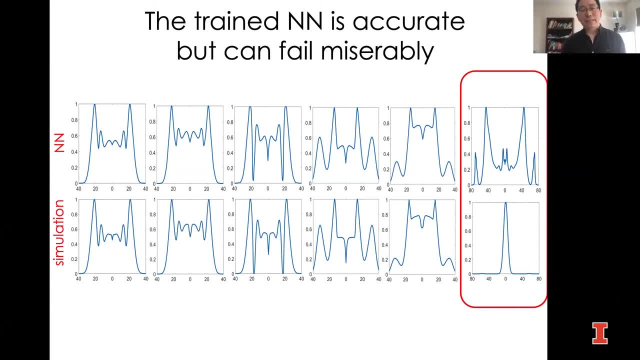 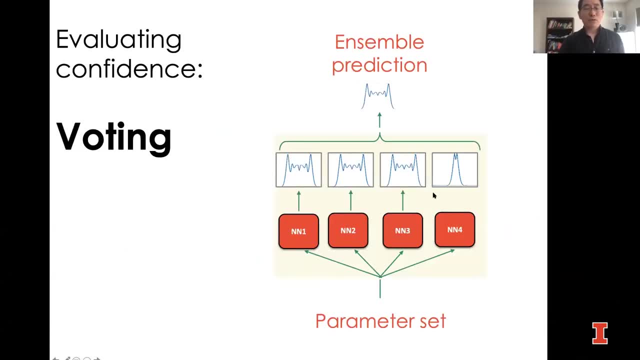 If you were to do that, you're defeating the purpose of using the neural network, right? So what we decide to do is to use a very simple strategy, is to do ensemble prediction. So the notion is that, given the same parameter set- I should say the training set- I will train four. it doesn't have to be four, just multiple neural networks independently. 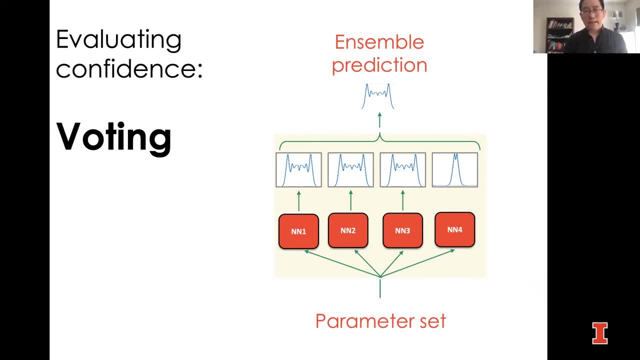 Of course the training process has intrinsic randomness, depending on how you initialize different neural networks right And when I do the training right, every neural network can make its own prediction And then we just check the consistency, like the voting result. 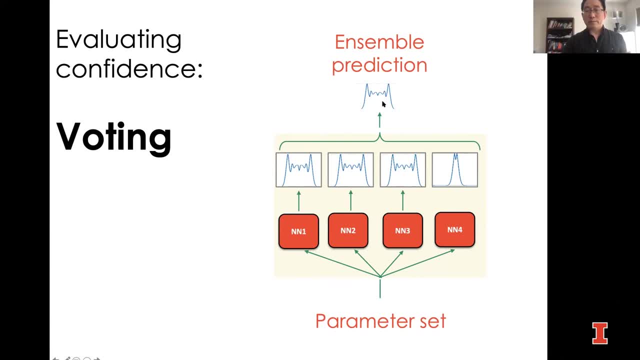 So in this case, like the majority is predicting this, I can use this as an ensemble prediction. More critically, whether these predictions are consistent or not consistent will give me a metric on how confident the predictions are. So we actually check that right. 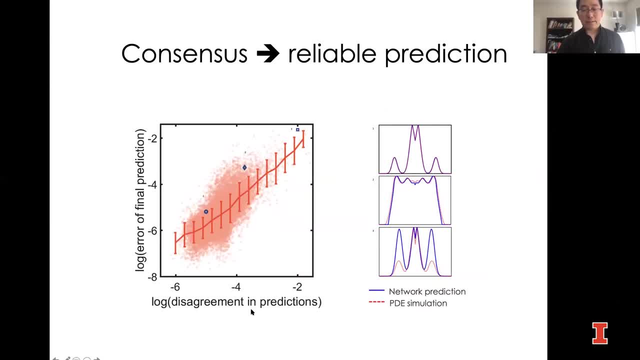 The idea is here. this is a disagreement between predictions made by the neural networks. How much they disagree with each other. And this y-axis is a difference between the neural network predictions from the ground truth which is simulated by the mechanistic model. 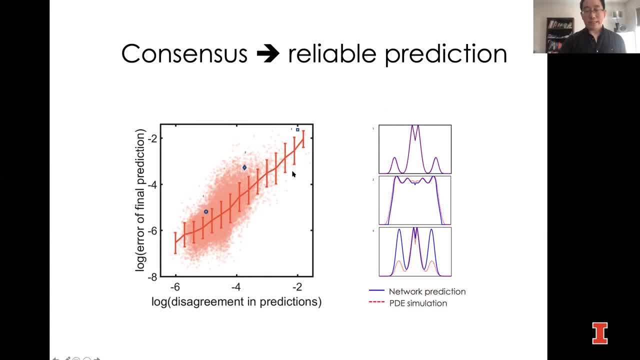 You'll see a very strong positive correlation. So the basic idea is that if the neural networks agree with each other, it's more likely to be a reliable prediction, But if the neural networks disagree with each other, then it's less likely to be reliable. 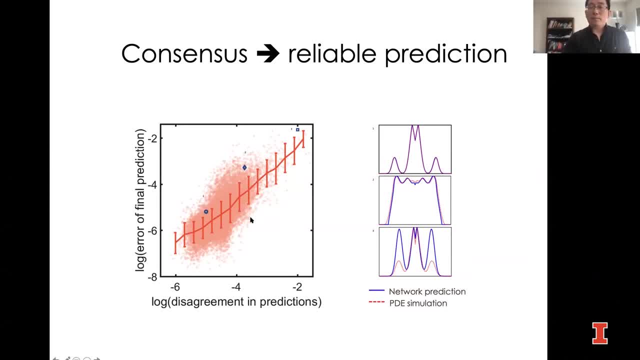 So you, as if you are doing this prediction, you get to set where you want to have high confidence in the production, right, Like in this quarter. it's very, very accurate for most of the examples. This is actually, I realize this is. this corresponds to that one. 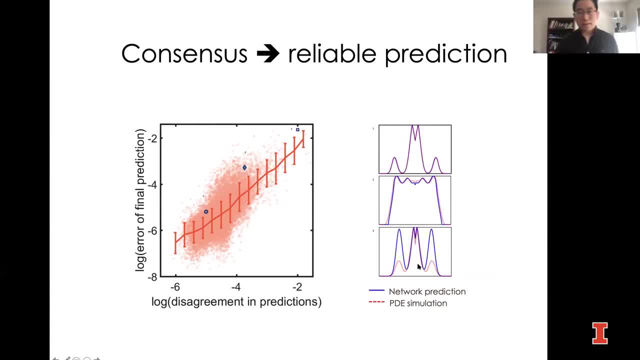 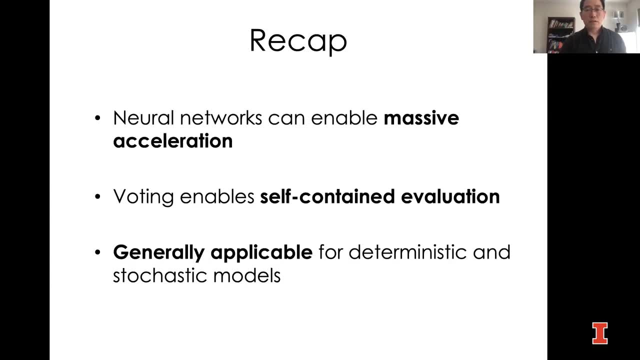 This corresponds to the bottom right, So this provides an intrinsic metric for us to evaluate how reliable the predictions are. To recap, this is a very basic, simple concept, Which is that neural networks can enable massive acceleration in predictions. You can always check to what extent the neural network predictions make sense by actually looking at the corresponding mechanism-based models. 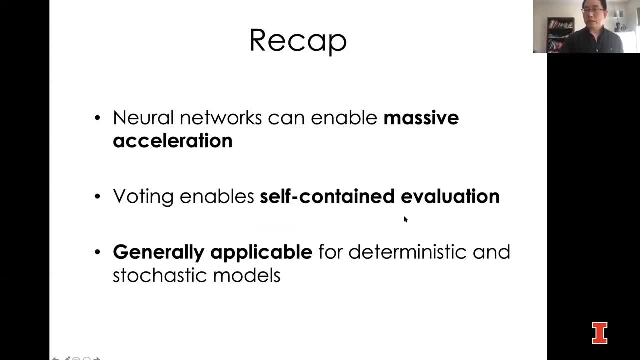 And voting actually enables self-contained evaluation of the quality of the prediction. We also demonstrate that this is generally applicable for some other models, including stochastic models You want to use in a context where the simulations are very time-consuming, such that you can gain. 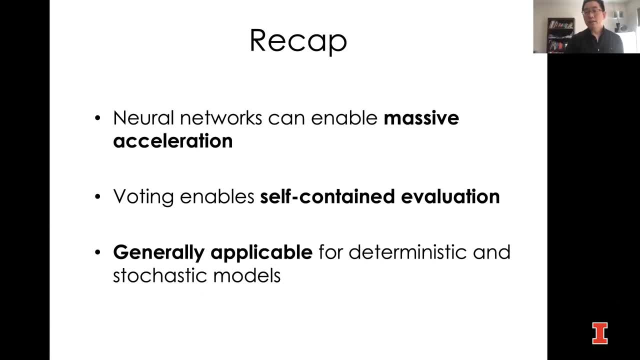 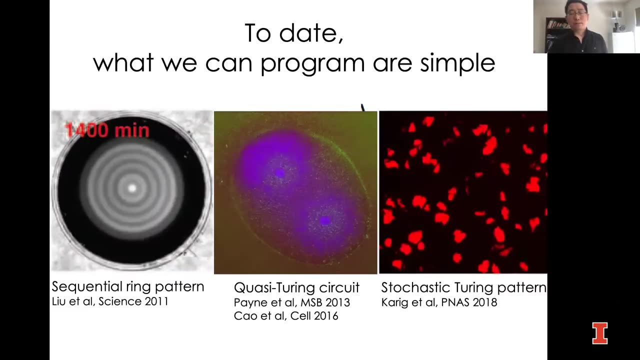 But on the other hand, it's not so time-consuming. you won't even be able to generate sufficient training data, And the latter is actually quite a challenge for some of the examples we're trying to tackle. Now, coming back to the challenging programming pattern formation. 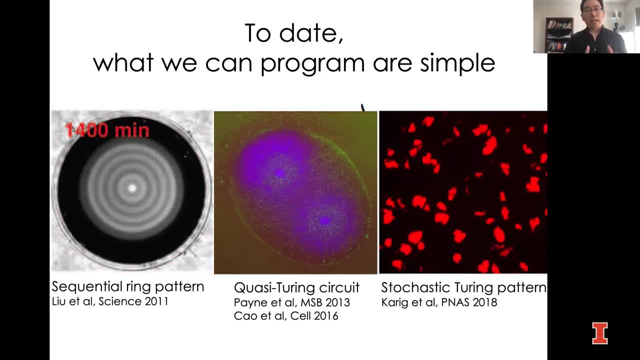 Today I mentioned, there are only a limited number of examples of self-organized pattern formation, including a pioneering work from Chen Li Liu, who is now in Shenzhen Institute of Advanced Technology. It's sequential ring pattern formation, So this is one I just described briefly. 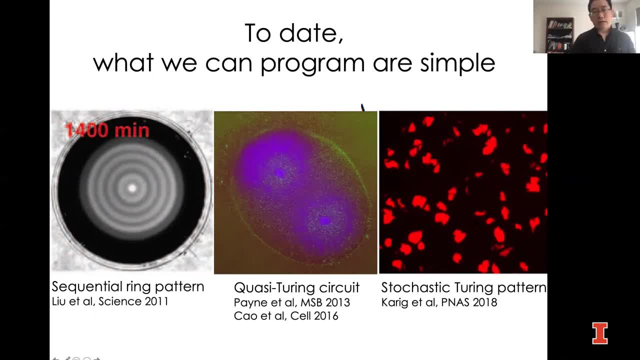 And also a wonderful example, I think, and is involved in right And Dave is correct, and both of whom I know very well, Coming out of Ron Weiss's lab, right Stochastic Turing pattern. If I look at one of these patterns, 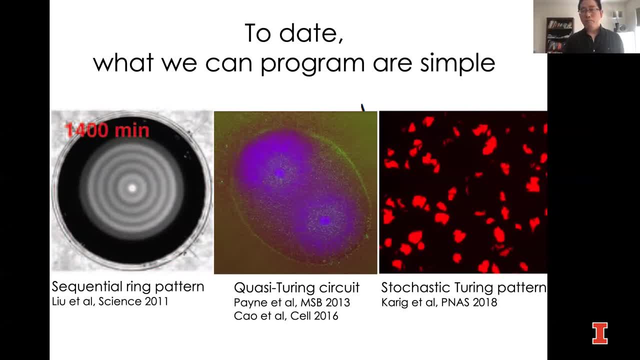 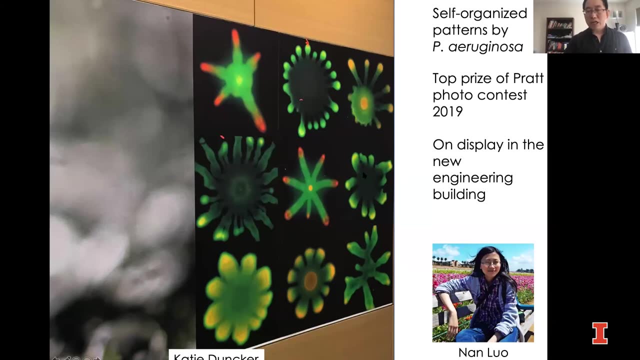 they're relatively simple In comparison to nature. our ability to generate more complex patterns, indeed, is very, very limited. Here's a lot of example. This is just simply a picture taken by microscopy, picture taken by a current postdoc, Lan Nuo. 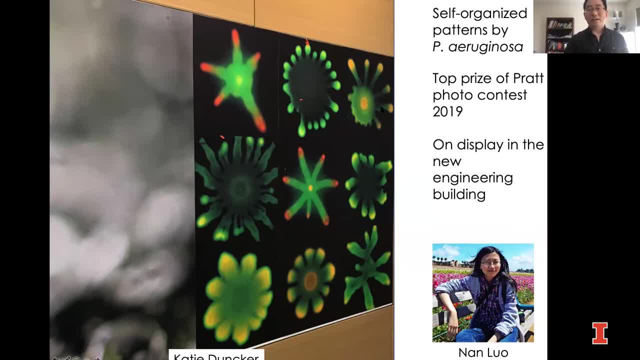 And it's very, very beautiful. This is generated by a model organism called Pseudomonas aeruginosa. It's an opportunistic pathogen, But here we're only focusing on the pattern formation capability. It actually won the top prize of the Pratt Photo Contest. 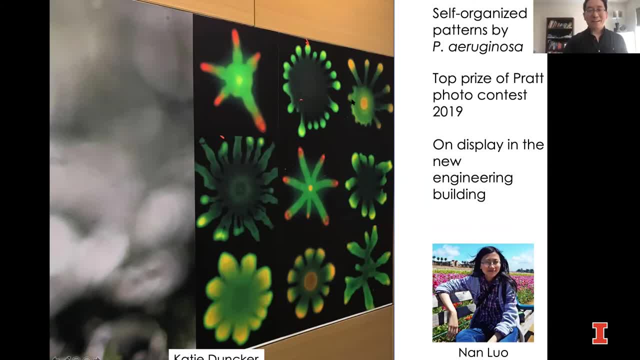 a couple of years ago And now it's on display in the new engineering building, And this was taken by another grad student of this photo on display. It's gratifying to see that people actually appreciate the beauty in the scientific data. This is what we try to understand. 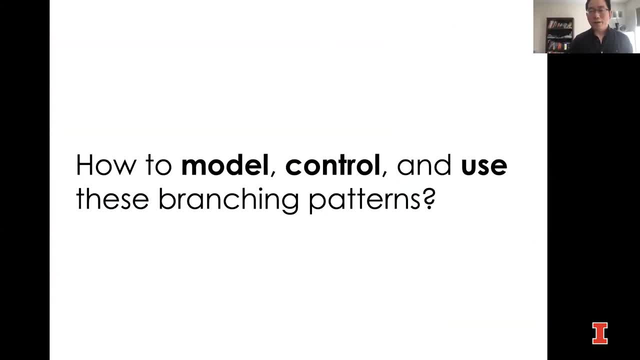 So the question we're asking is how do we model and control and use this sort of branching patterns? I mentioned that the patterns we can program are relatively simple, not limit the possibilities of different applications we can think of. So the somewhat basic question we are asking is that: 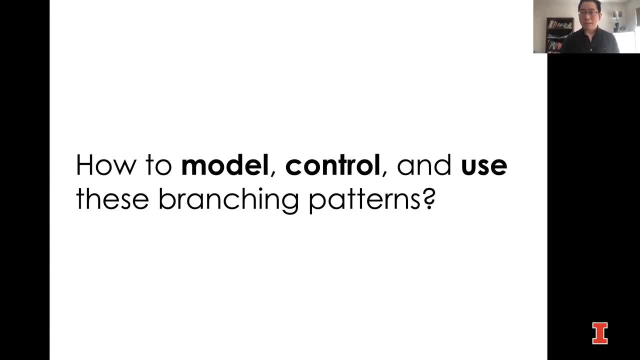 if I have the ability to generate much more complex patterns, then maybe I can think of more diverse and more interesting applications going beyond the pressure sensor right. This turns out to be a very, very difficult problem, much, much more difficult than we initially anticipated. 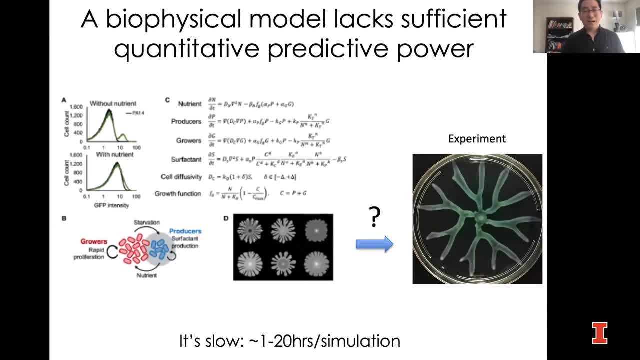 We're not the first to look at the branching patterns. It has been looked at for many years And the typical approach is to build a biophysical model or reaction diffusion model. I'm not going into details of this To look at the conditions where you lead to the emergence of the patterns. right, 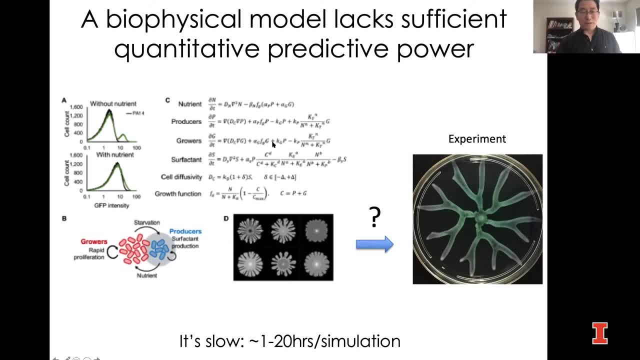 And here it's like we generate this model that generates the emergence of the patterns. In that regard, it's good, It's consistent with what people have generated in the literature, But qualitatively speaking, we're missing out of some very important features. 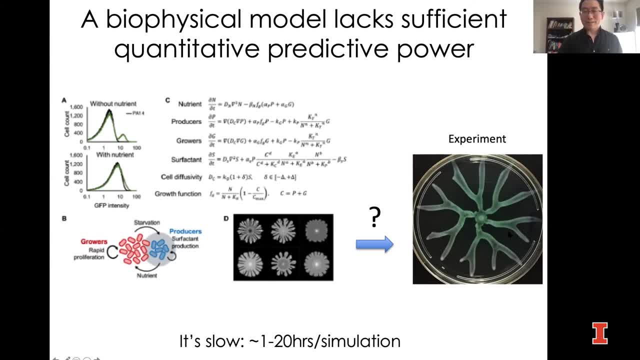 of the patterns we see in the experiment right, And the quantity of agreement is not great. For instance, in the experiment we tend to see the branches can be very, very thin right. Along each branch the width tend to be approximately constant. right. 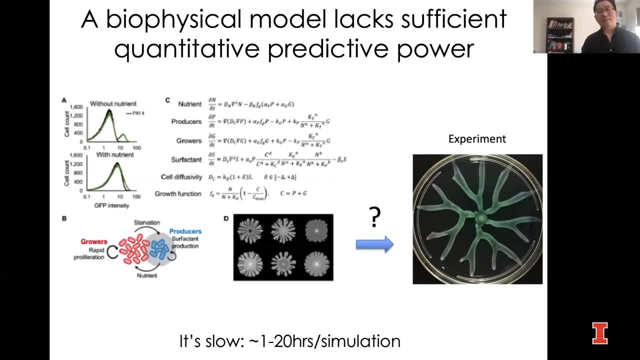 And we tried many, many different formulations. It's incredibly, I would say, depressing. It's even depressing to me, right, Multiple years. And what's most depressing is that when we look at this sort of modeling effort, when we see a disagreement that we cannot feel, 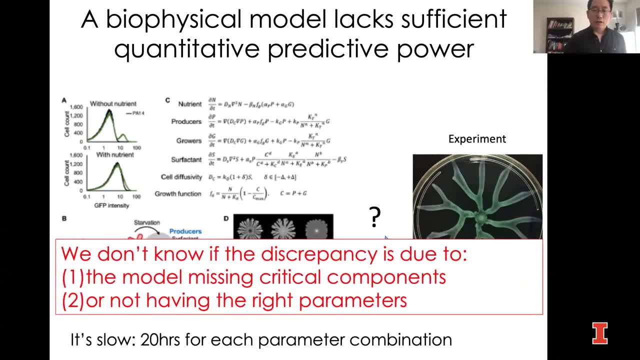 we actually don't know what's wrong. We don't know if the discrepancy is due to the model missing some critical components. Or, for instance, I could write down one equation formulation: knowledge, but if it's not in the right form, then there is no hope, right? 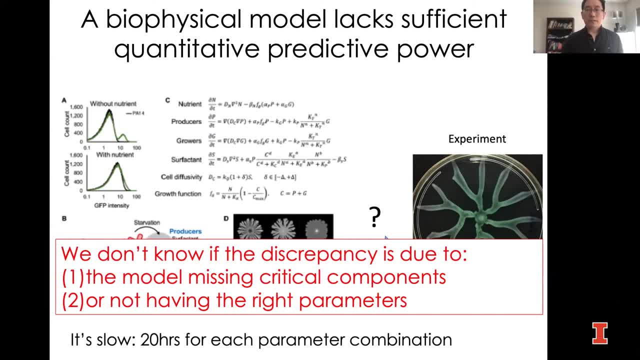 Or even if the model is in the right form, there may be parameter space we simply technically cannot fully explore. We're not in the right parameter to map. We actually don't know why. which case this corresponds to right, Because every simulation is very, very slow. 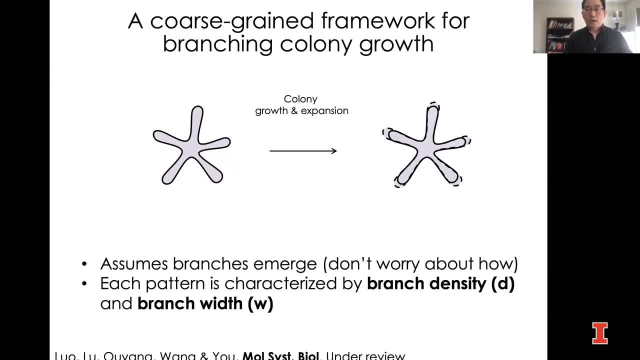 Very, very slow. Instead, we want to take a step back. ask the question: can we find a larger way of describing the patterning process that will enable us to make reliable and biologically relevant predictions? So the approach we're taking is more extreme coarse-graining. 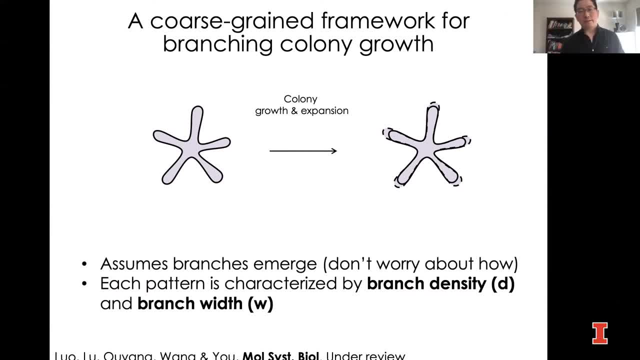 We ask the basic question. let's assume the branches can emerge. We don't worry about how right, We just assume they can emerge Based on the observation. right, these branches are typically constant width. right, We assume every pattern just characterized by two parameters. 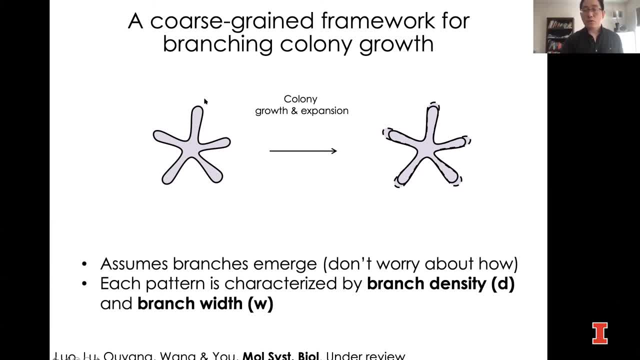 branching density and branching width. Of course, when the cells grow, when the columns become larger, there will be additional branching- and to maintain certain degree of branching density- By branching density I mean how many branches you have per unit length, right? 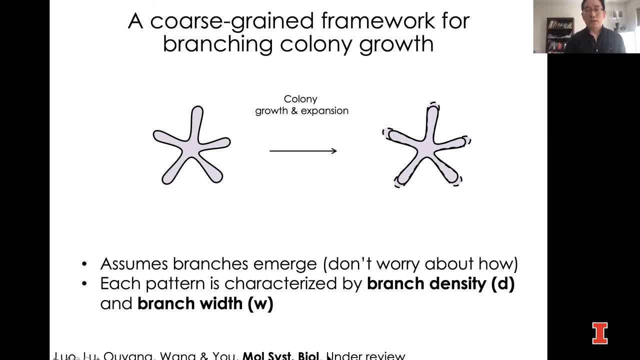 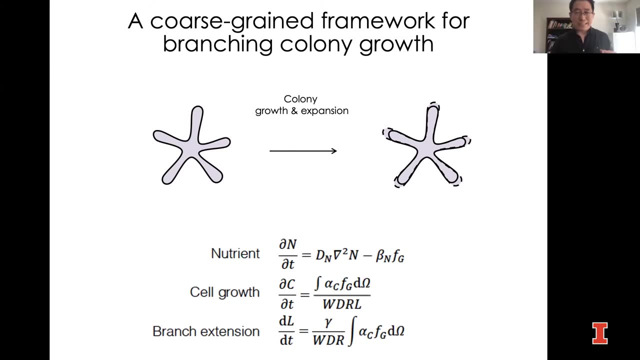 So this paper is actually almost accepted. I think the reviewers really like it And these are pending some minor edits in the text, right. So this is kind of an advertisement of a paper to come out. So if we take that approach, turns out that we can use a very simple model. 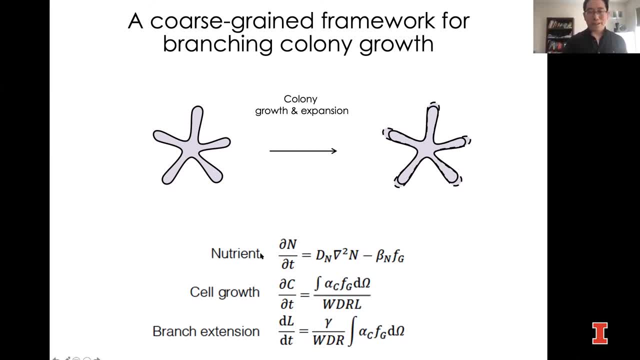 where we still model the nutrient, like using the reaction-diffusion equation, where this is a consumption, this is diffusion right. For the other components we can model actually use ordinary differential equations. Ordinary differential equations: You have the growth and have the extension right. 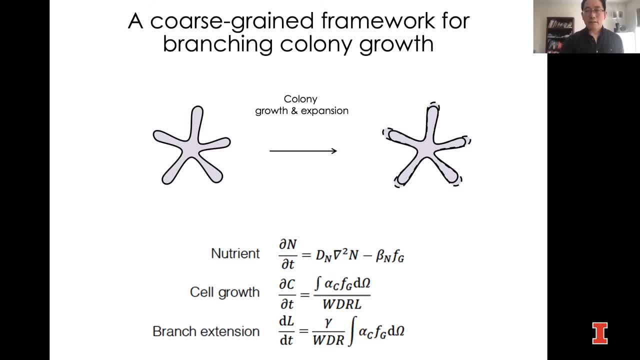 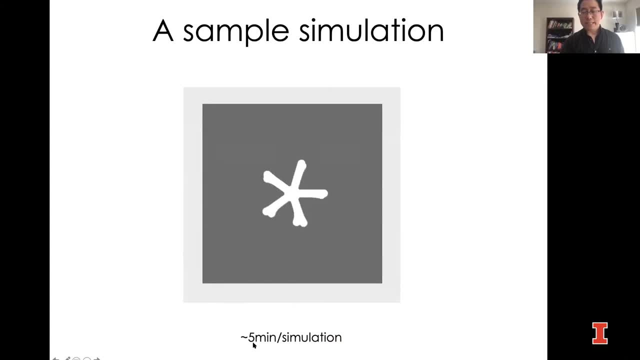 Then we ask: using this simplified formulation before I go into that, so this is a sample simulation. I want to emphasize this is what are some magnitude faster than the PDE model. I actually generate characteristics which are agreed much, much better. 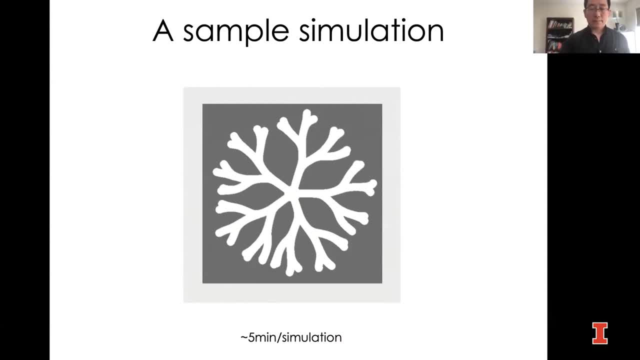 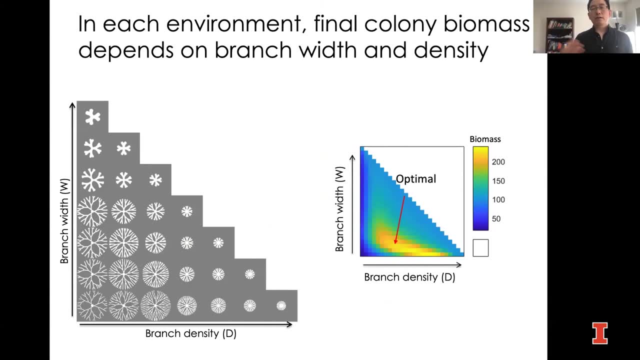 with the experimental data, with the experimental data. So, using this model, we're just asking a basic question: How does the overall system or the overall system output, in addition to patterning how the overall biomass depends on these two parameters- Turns out in each growth environment? 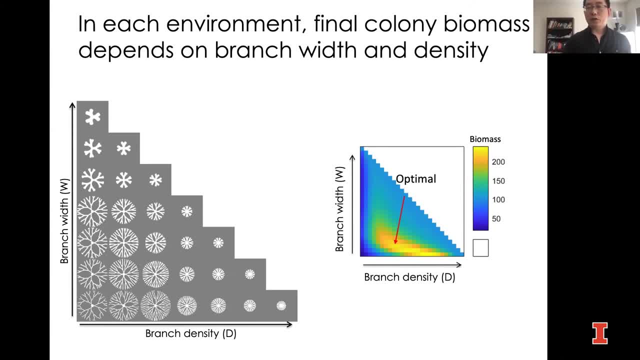 so in our simulation that's set by the amount of nutrient that's available. The colony biomass accumulation depends on branch width and density. Showing here is actually the patterning process. If I increase the branching density you see much, much denser branches. all right, 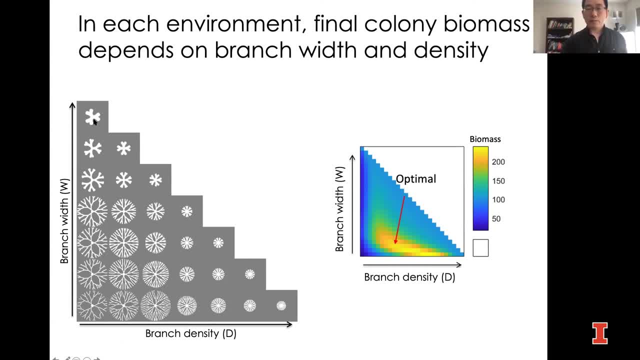 If I increase the width, they have thicker and thicker branches. Above this line is when these branches start to overlap with each other. You don't have any branching anymore. It's just a circular colony, right, And we can quantify with higher resolution. 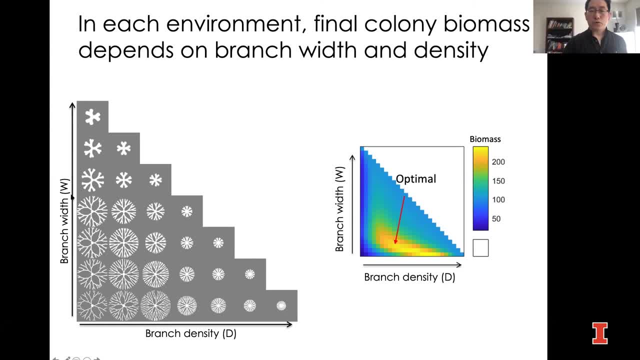 of the biomass as a function of these two parameters. What's interesting is that for a given environment you will actually have optimal biomass accumulation for some sort of intermediate width and density. Then we ask to what extent this optimal growth would depend on different growth environments. 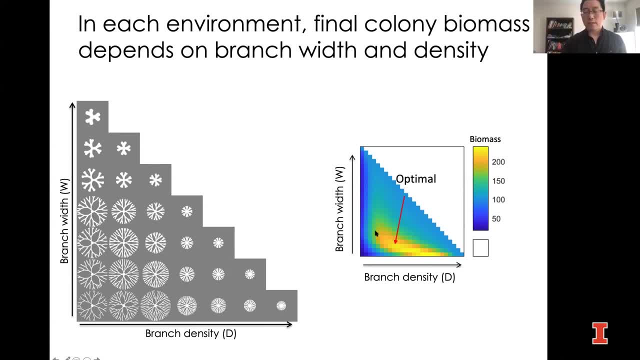 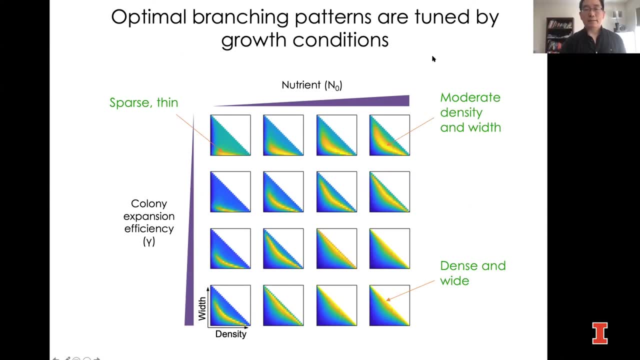 So how does this shift according to different growth environments? Indeed, that's tunable outcome. So the optimal branching densities are tuned by the growth conditions. There are two ways we can tune the patterns and the growth. One is controlling the amount of the nutrient. 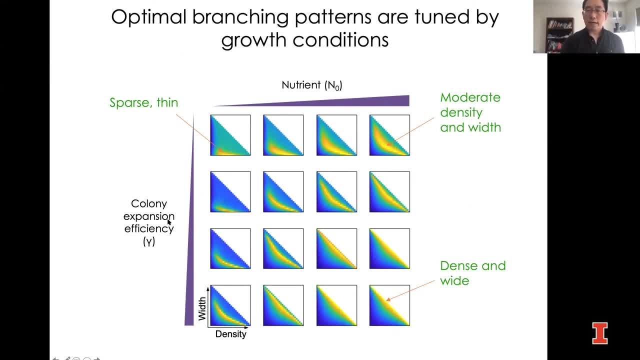 One is to control how fast the cells can move around, which influence the branching, the colony branch extension speed, right. The key point I want you to focus on is the yellow portion that shifts according to the nutrient environment. When I have increased the nutrient, 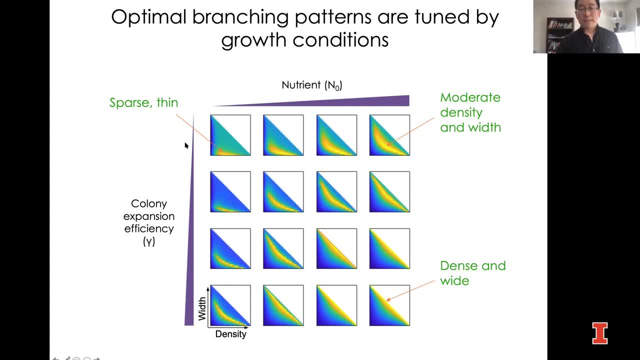 while fixing the mortality, I will see increasingly the optimal patterns to have increasingly denser and wider branches right. And if I increase the mortality of the cells by reducing the agar density I will tend to have much more dense branches. So these are all shaped by the growth conditions. 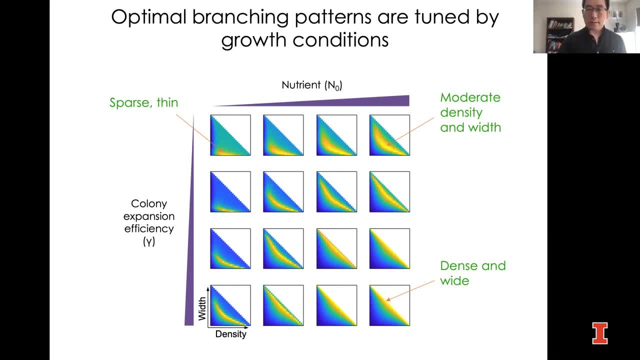 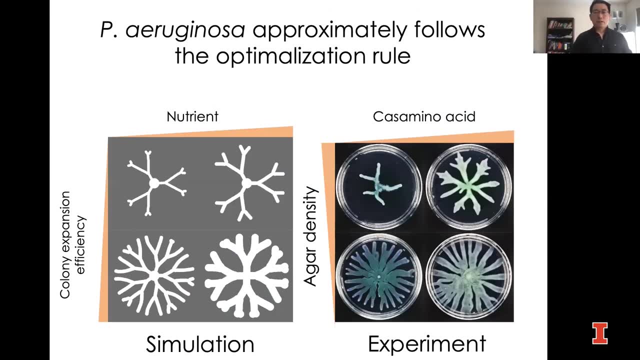 These predictions are actually consistent with how pseudomonas respond to these growth perturbations. So, in other words, pseudomonas appear to approximately follow this optimization rule that if I increase the nutrient concentration, this is increasing the decrease in agar density right. 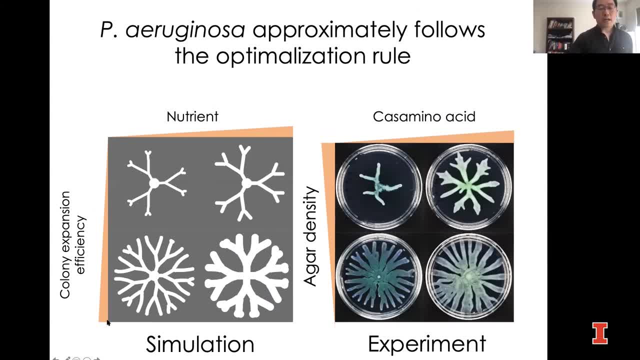 Decreasing the agar density, increasing the colony expansion efficiency. So these are the numeric predictions And these are actually experiments. There are much more extensive experimental data to validate the consistency between the modeling and experiment. So the key point is that the pseudomonas appears to approximately 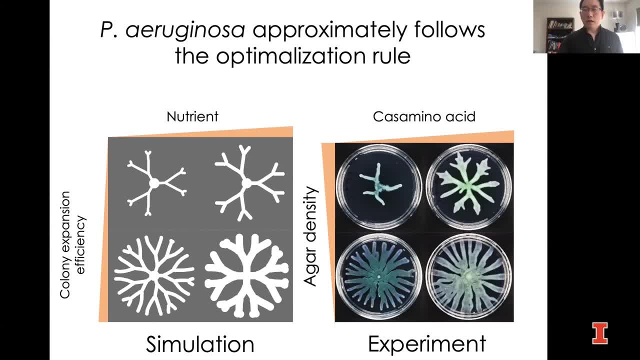 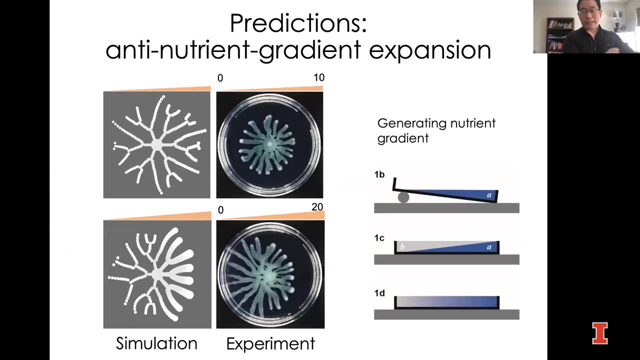 follow this optimization rule Now, given that we can actually take advantage of this property and make predictions of the pattern formation of pseudomonas under different conditions. One example is actually very intriguing is that pseudomonas can have this anti-neutron gradient expansion right. 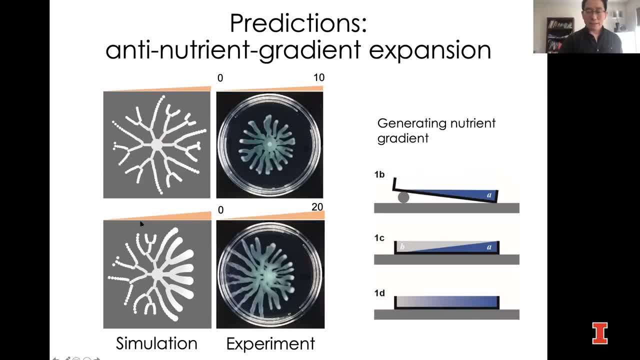 This is a prediction, If you have. in this case you have a gradient. there's a higher concentration of nutrient on this side, neural nutrient concentration on the left-hand side. The branching actually extends more on the left-hand side, right. 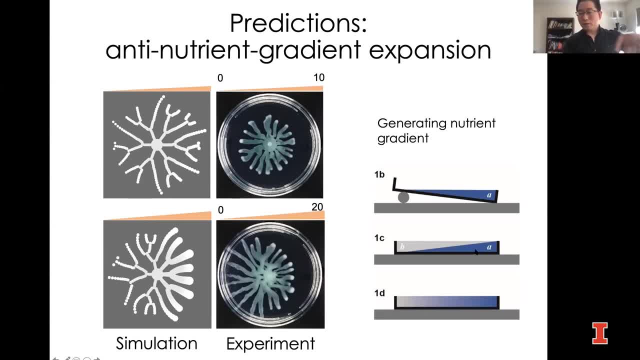 And this is experimental data. In the experiment, this is how you can create a nutrient gradient: by generating the agars: one containing the nutrient, then you pour the agar without the nutrient, So you can create this nutrient gradient. This turns out to be non-trivial behavior of the system. 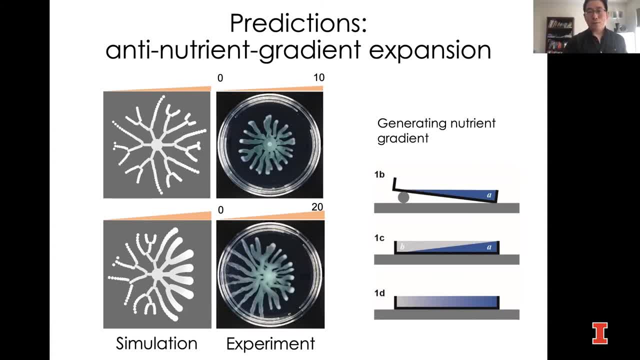 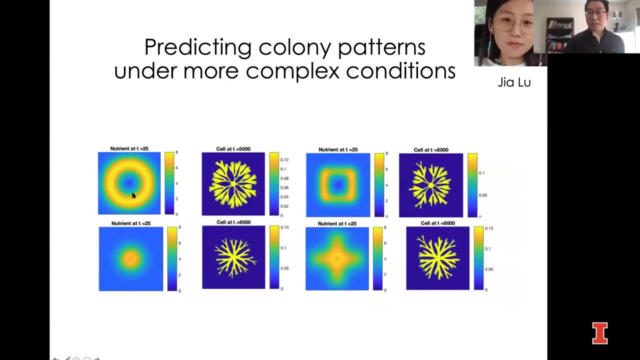 that the model actually can capture. Of course, you can predict more sophisticated scenarios, And these are the predictions of how the branching pattern is going to respond to the growth environment. You can think of this as another way of controlling the patterning process. 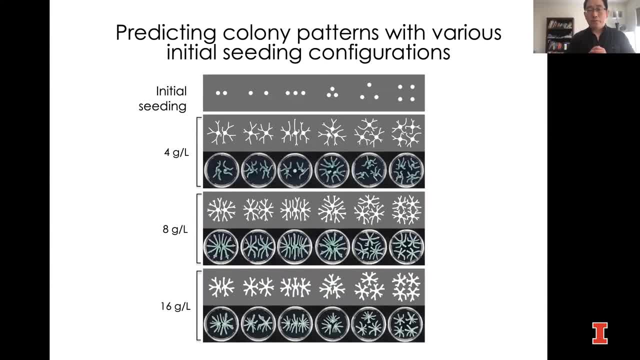 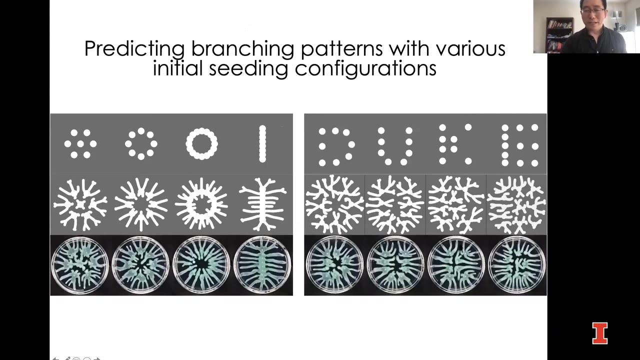 Patterning process, Or you can predict the colony patterns with various initial seeding configurations. So in every case, the model is doing a terrific job in terms of predicting the outcome. that's consistent with experimental observations. Well, there's more. There's just very beautiful pictures, right? 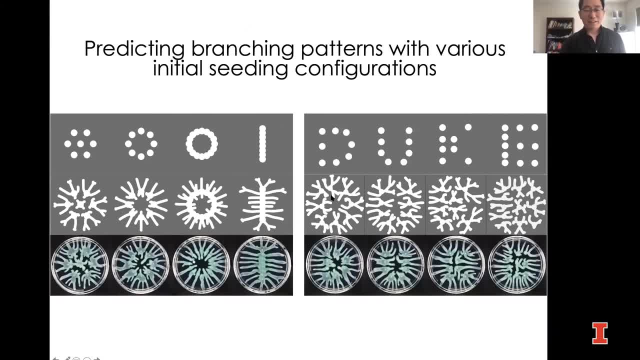 And these are the initial seeding patterns, And these are the model predictions And these are the actual experiments. Well, now, coming back to the point, now we're developing the capability of predicting and explaining these sort of patterns. So how do we want to use these patterns? 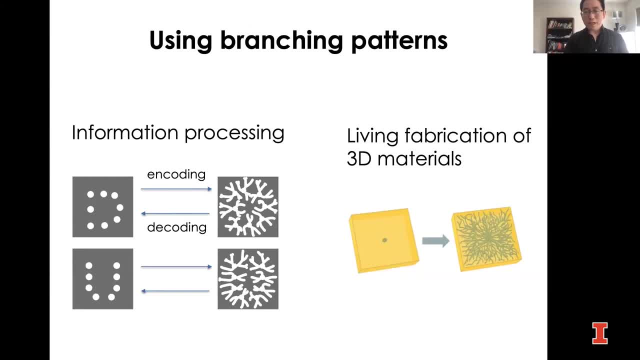 We have ongoing research. Now, if we have these abilities, we generate these sort of patterns computationally and experimentally. One question is essentially using biology for us to compute The notion is that the pattern generation process can be considered as encoding process. 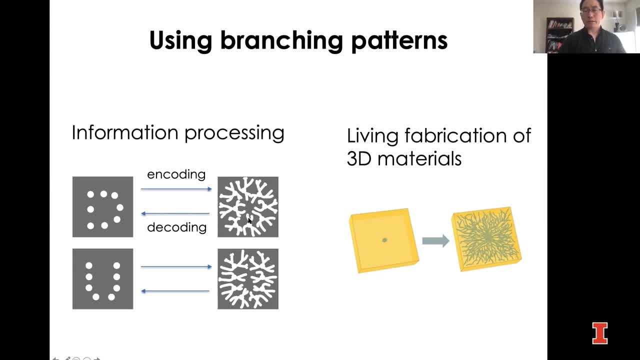 If you have certain initial configuration, you generate the final pattern. That's information encoding. Now, starting from this side, if I can deduce my initial configuration, then that's a decoding process. Decoding process. So in ongoing work we're trying to explore. 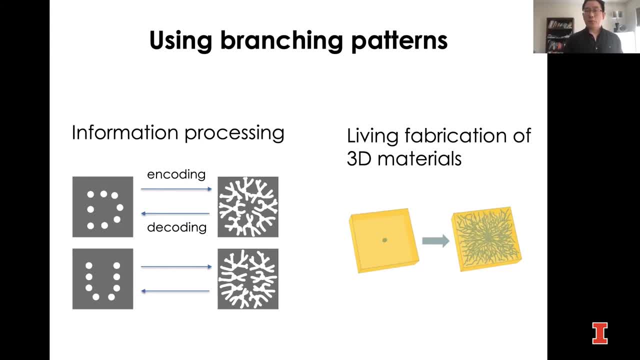 to what extent you can utilize self-work as pattern formation, as a way to generate this information, encoding and decoding in a robust manner. A lot of aspects we're interested in in collaboration with some of our colleagues in the materials engineering, is that, if I can control. 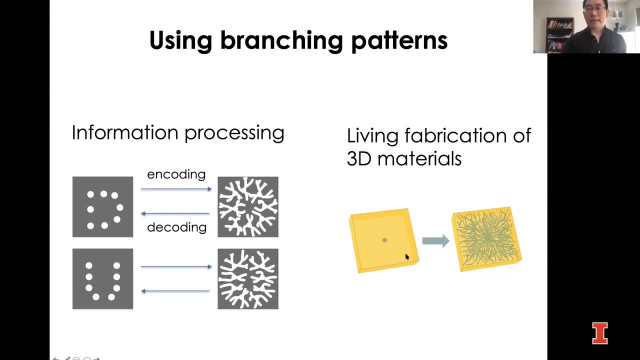 this sort of branching pattern process. if we introduce the right effectors, then can we generate this sort of branch materials which could have optimal optimized transport properties for different applications. right, These are the potential applications we're currently exploring. Now coming back to the notion. 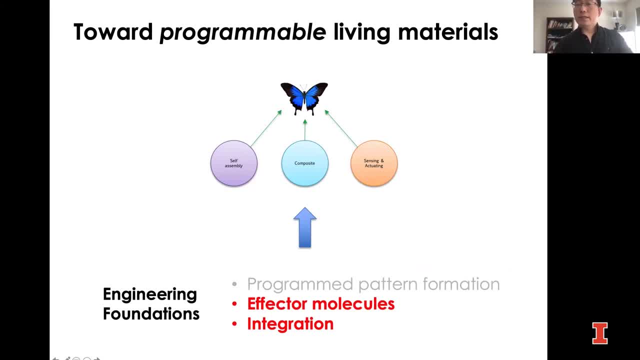 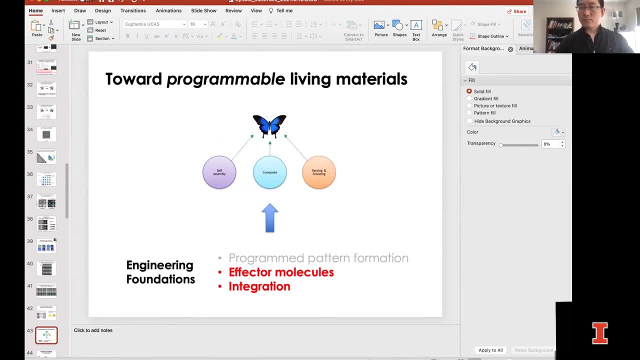 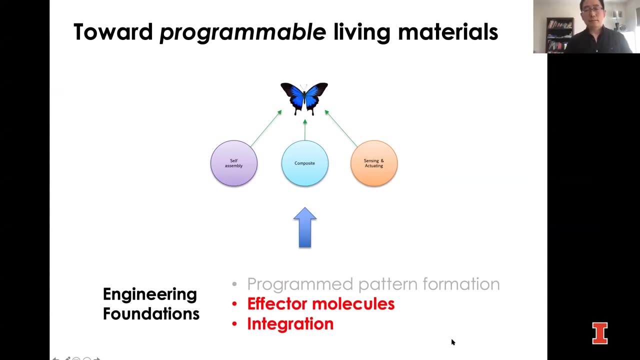 of leaving functional materials. let me check if I have 10 more minutes, Is that right? Yeah, Okay, thanks, That should be sufficient. The other aspect we're exploring is how do we integrate and generate actually functional devices by combining engineer cells. 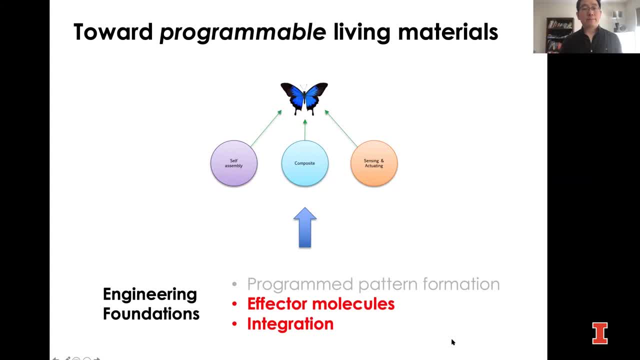 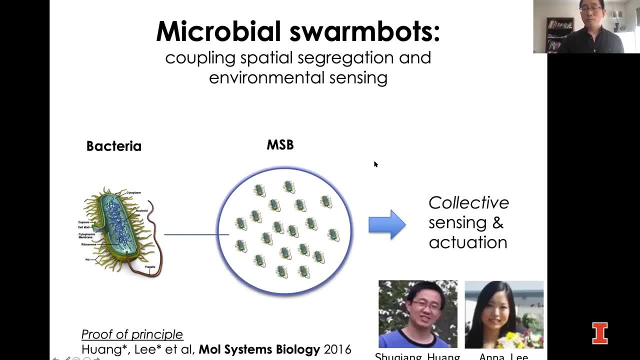 and with stimulus, responsive materials. So this alliance line of a platform where engineering, which we call microbial swan bots- it's a loose term- The key point is to couple spatial segregation and environmental sensing to generate well-defined functional devices, right? So the idea is that we have engineer bacteria. 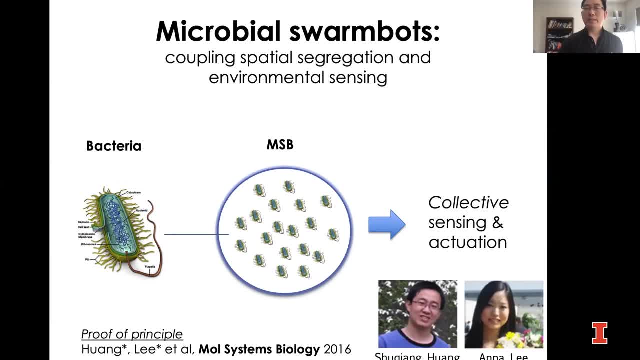 with certain types of sensing actuating capability. We encapsulate groups of these bacteria and this provide a well-defined interface for the group of bacteria to carry out their function. So we'll want to realize collective sensing or actuating functions. The proof of principle was done a few years back. 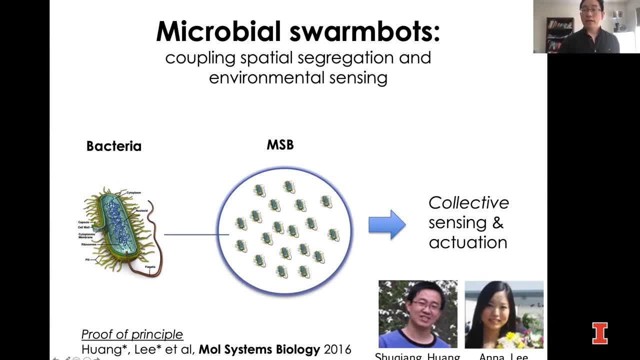 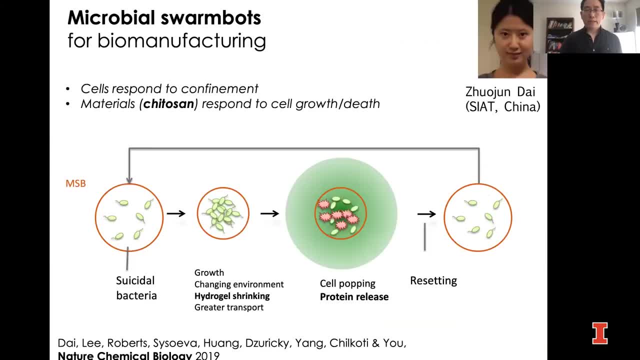 Right, Demonstrating how you can program well-defined functions in this format, And this is like the second generation, where we engineer the bacteria. They can sense the spatial confinement. We also chose a material that can respond to bacterial growth and death, In this case. 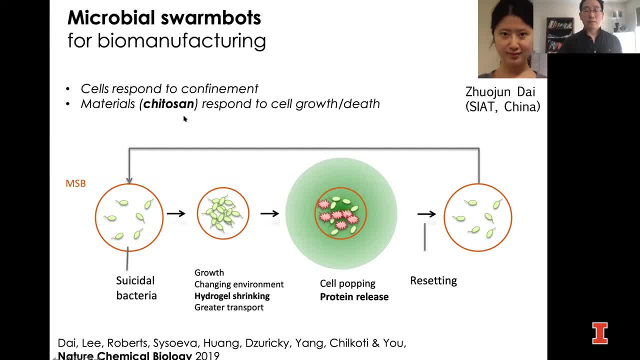 it's a very common and biocompatible material, chitosan. right, Here's a basic operation of this device. You have engineered suicidal bacteria. Now they can pop open at high enough density and we encapsulate them. They will grow, right. 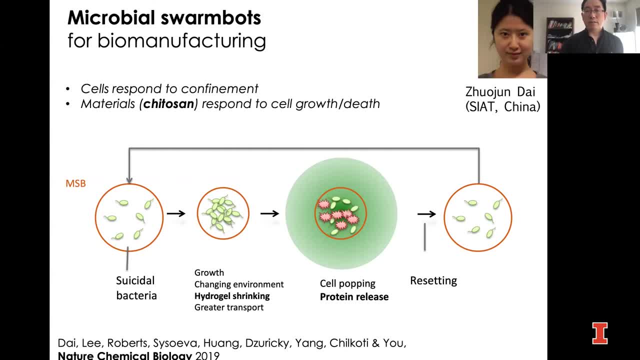 As they grow, they are going to change the chemical environment, For example, changing the pH and ionic strength. So in response to this changing chemical environment- what's really interesting, this is just the property of the chitosan: the chitosan will shrink. 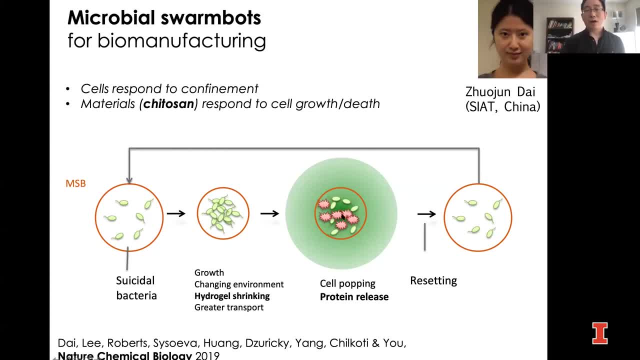 And this shrinking process turns out roughly coincides with the popping of the cells. So, in essence, you create a hybrid device where the cells grow and they're going to pop and the material is going to shrink and squeezing out the content produced by the cells. 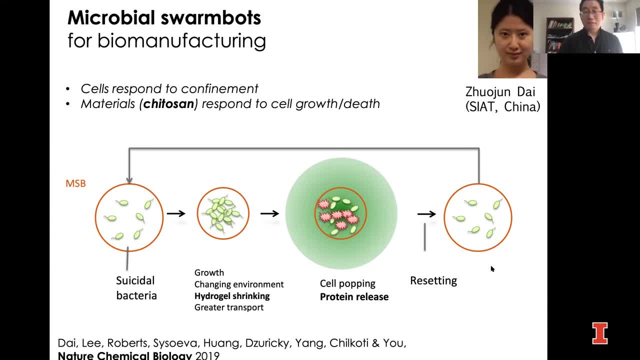 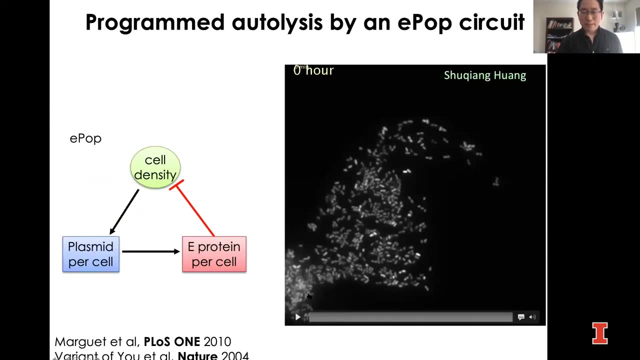 When the cells pop, they release their protein content And you can use this as a integrated separation device. right, You can reset this process, keep going and produce and fabricate proteins. So here is a basic building block. This was a circuit we built a few years back. 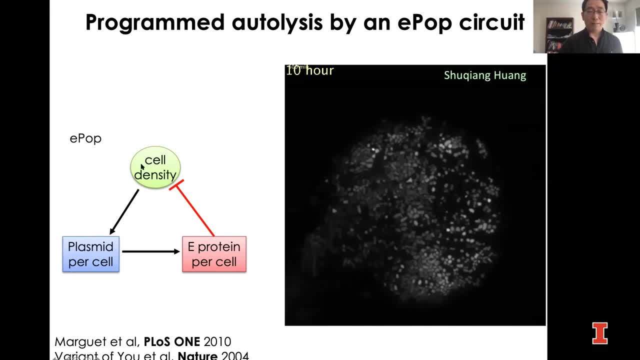 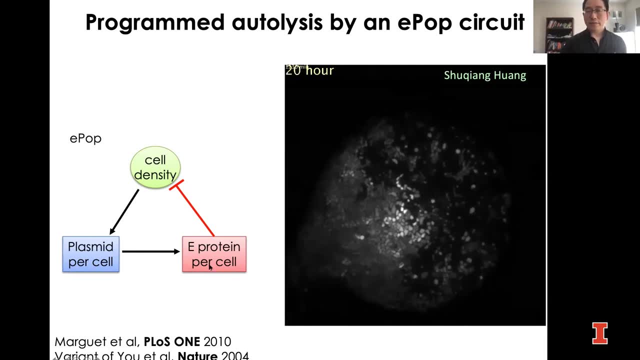 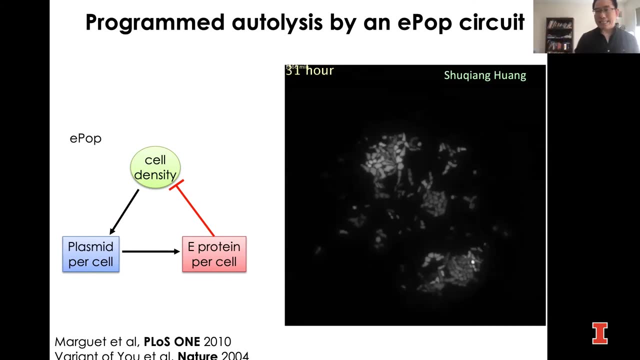 This circuit. logic is very simple. We call it EPOP. You have high enough cell density will lead to higher copy number of the plasmid, leading to higher gene expression of a toxin, E protein from 5X174, which blocks the cell synthesis right. 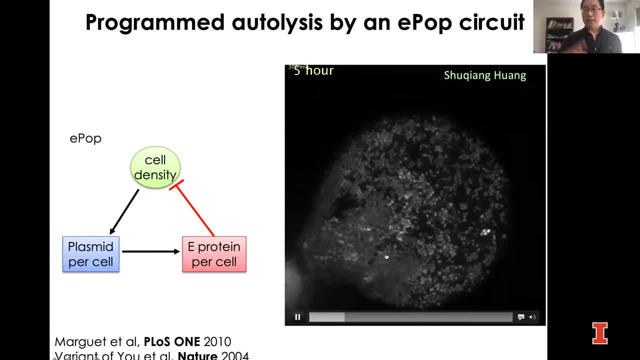 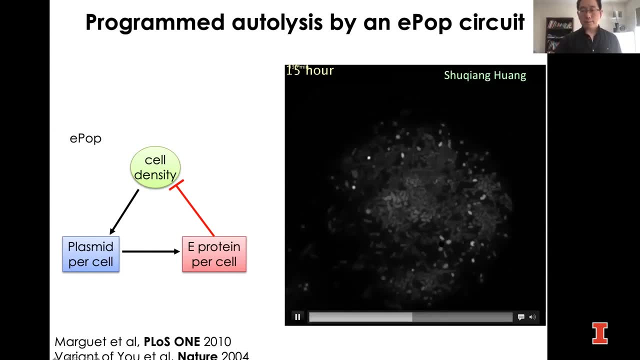 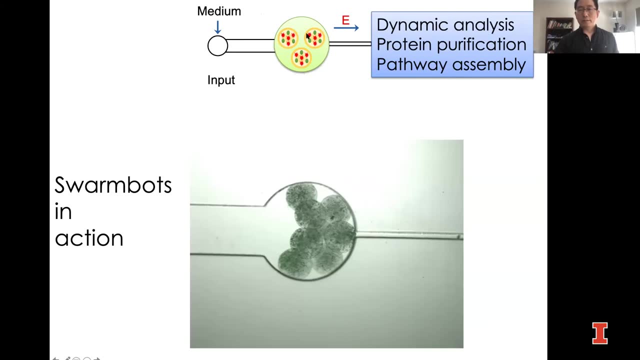 So, as a result, you will see the population level oscillations due to this lack of feedback control right Now. if you integrate with the SwamBot platform. now, this is the microfluidic device we use to quantify this response, This SwamBot template here. right, 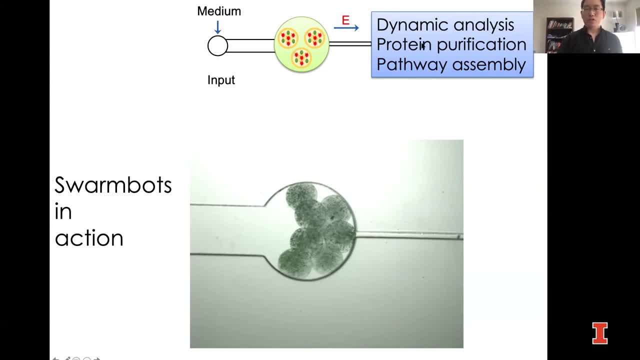 This is where we put in the nutrient, And downstream we can do dynamic analysis, protein purification and pathway assembly. So here is microbial SwamBot in action. So the nutrient flow in periodically. You'll see every time you flow in. 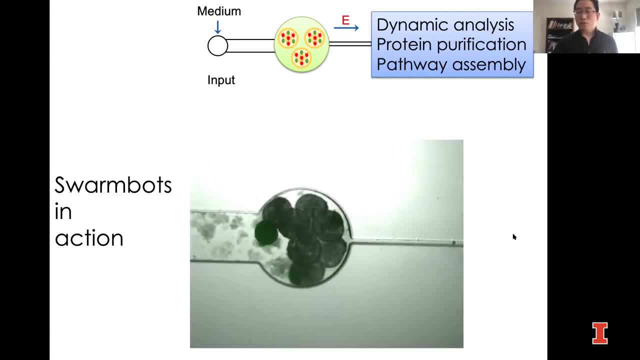 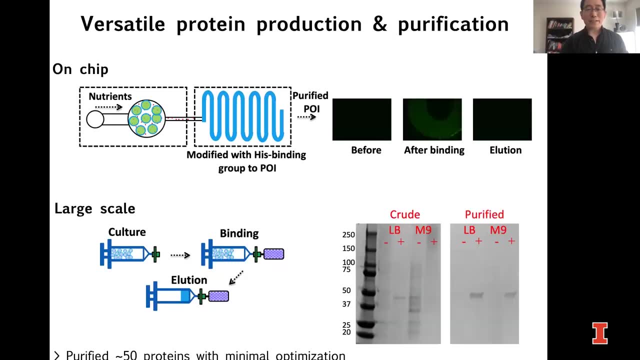 it's resetting the size of the SwamBot, right, And you can do downstream analysis and protein purification, et cetera, right. Here's one example. Well, here is just a brief explanation how we can couple this device with downstream processing to generate. 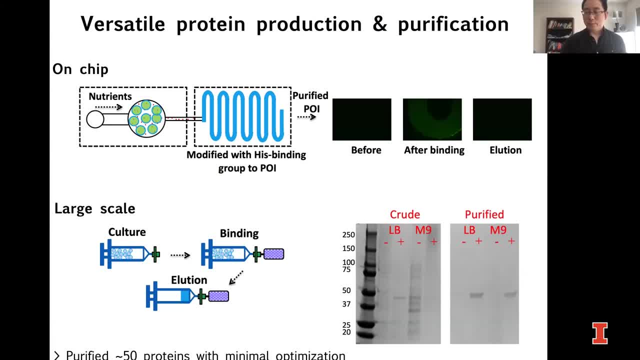 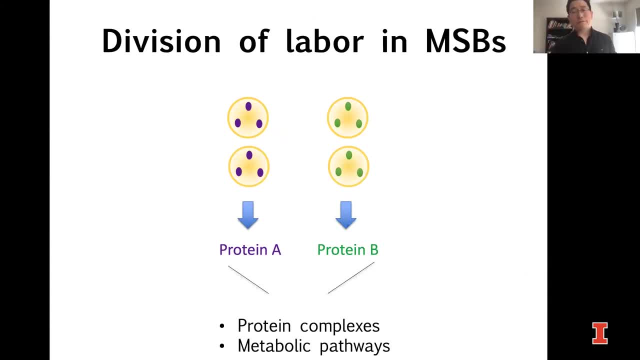 to enable versatile protein production and purification right. A larger aspect we are working on right now, which I find particularly exciting as well, is the notion of using this as a platform to realize division of labor. The notion is that, if I have one type of SwamBot- 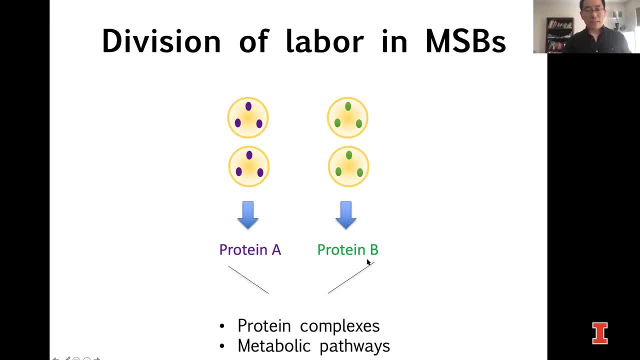 producing one protein, a larger type of SwamBot producing a larger protein. now you can form, you can control the stoichiometry of these two proteins. simply by controlling the ratio of these two types of SwamBots, You can generate different types of protein complexes. 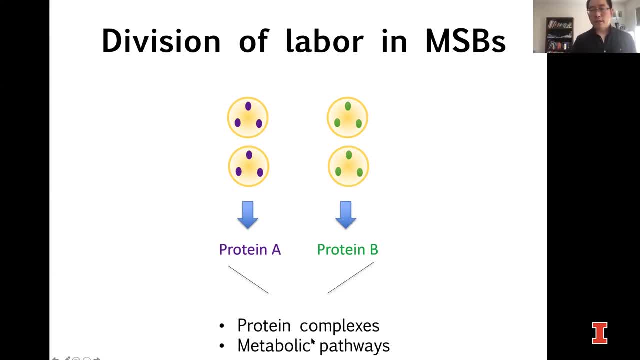 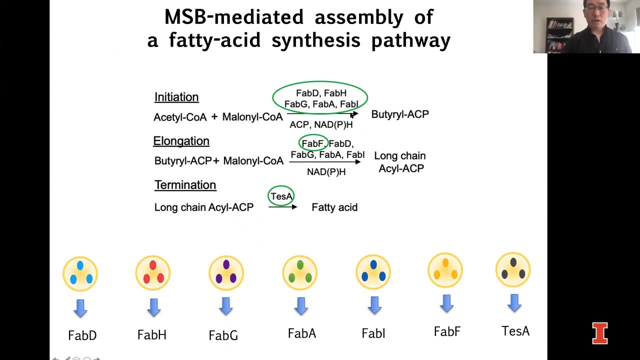 or tune the overall output of a metabolic pathway right. We actually demonstrated the latter as a proof of principle, We chose a well-characterized metabolic pathway just as a model system. This pathway requires multiple enzymes, right, Multiple enzymes. It's not important to remember what this? 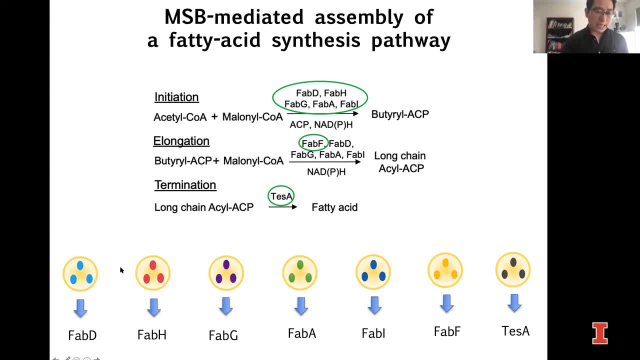 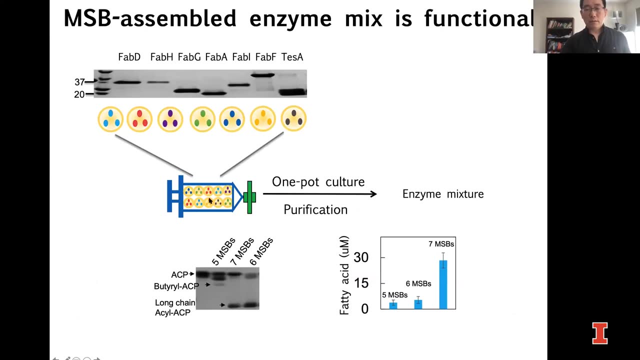 what of these enzymes are. It just requires multiple steps. That's a key point to keep in mind. We generate multiple SwamBots, Each producing and releasing one enzyme right, And then we put all of them together and generate one part culture. 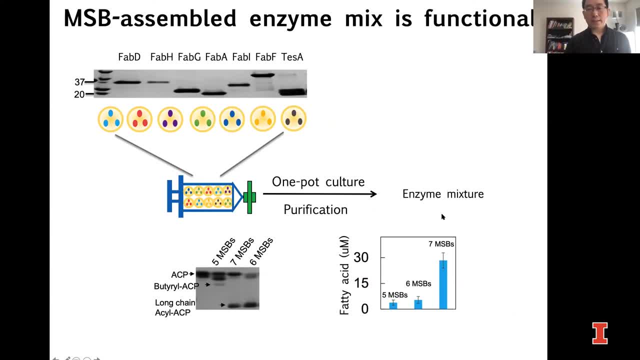 and then do the purification, Then we can directly generate the enzyme mixture And turns out this can directly reconstitute the metabolic pathway and generate the desired product. So this is a proof of principle of demonstrating using the microbial SwamBots to do. 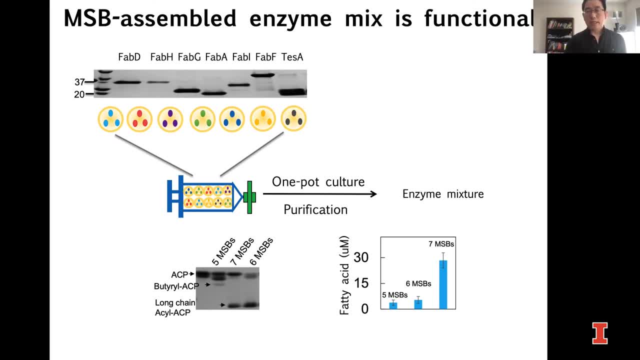 optimize, to reconstitute and maybe optimize metabolic pathway activities. Here we're directly using the enzyme mixture In ongoing research. what we're interested in is actually directly use the microbial SwamBots to control the metabolic pathway activities without doing the purification. 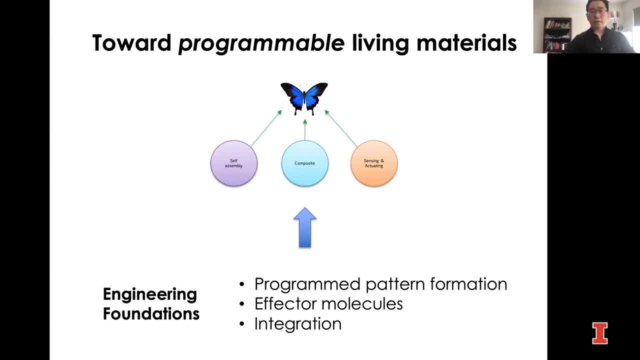 So this- I'm going back to this- essentially a summary slide. I give you a few examples How we think about programming, leaving materials, Addressing both of the fundamental bottleneck and also demonstrating some potential applications right. One aspect of research I didn't have time to go through. 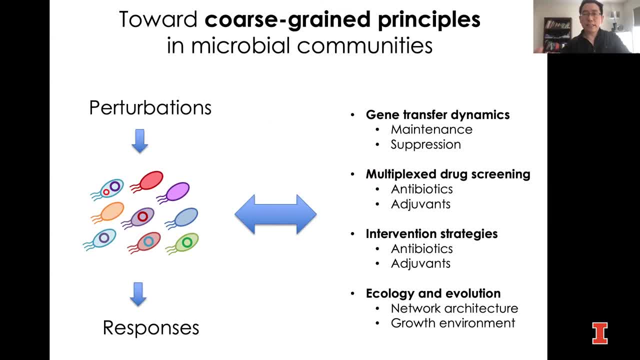 is facing a similar computational design challenge of high dimensionality is the dynamics of microbial communities, And the basic question- is the basic question we're trying to understand- is, given a particular microbial community, how does it respond to different types of perturbations? 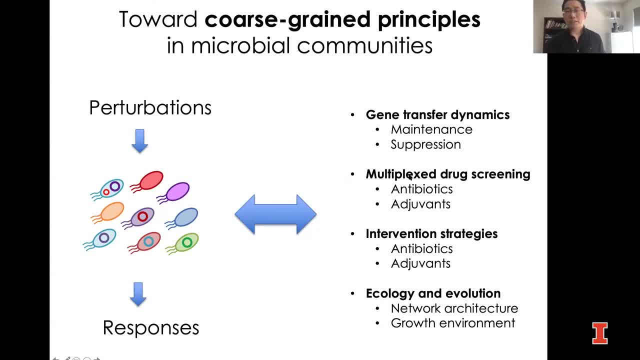 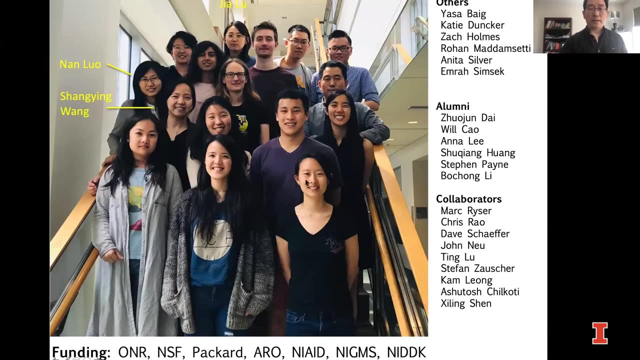 And under this umbrella, we're interested in gene transfer dynamics, screening drug responses and thinking about intervention strategies, and also basic questions of ecology and evolution. right With that, I would like to thank the people who actually did the work In this particular case. 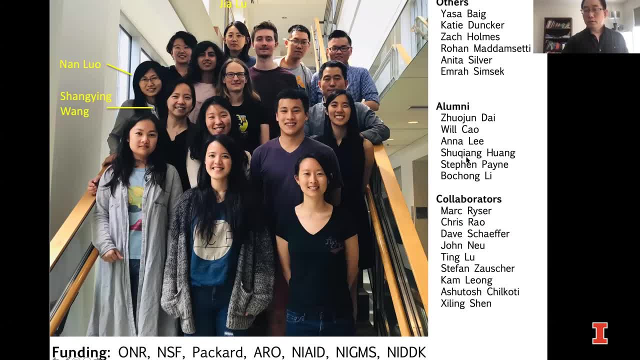 I had. the Patent Formation Project was pioneered by a few former grad students- right Primarily the work I had is Will Cao, and then a former lab member and a current post-doc landlord and grad student and the funding agencies. With that I'm happy to take any other questions. 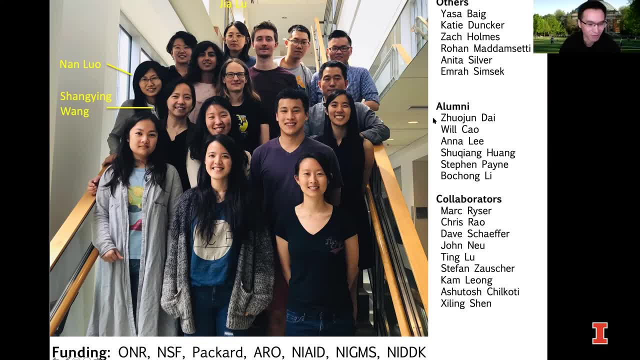 Thank you. Thank you, Lingcheng, for the very inspiring talk. Thank you very much. So it looks like we have a question right now in the chat. So how does the seed pseudomonas work with the two plasmids to generate others with a second ring and so on? 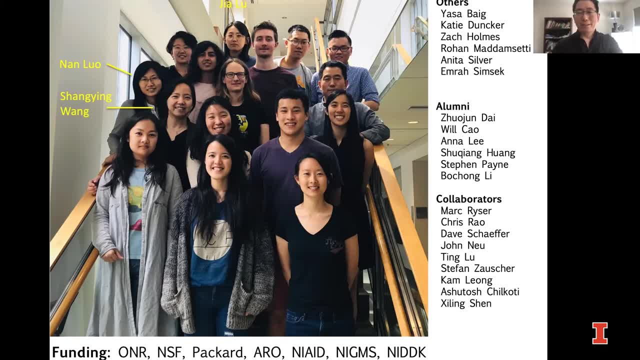 Oh, that's a fascinating question. We're still trying to understand or explain the branching patterns by the pseudomonas by themselves. We indeed are interested in how, if I introduce the ring pattern formation circuit into pseudomonas, that was actually initial motivation. 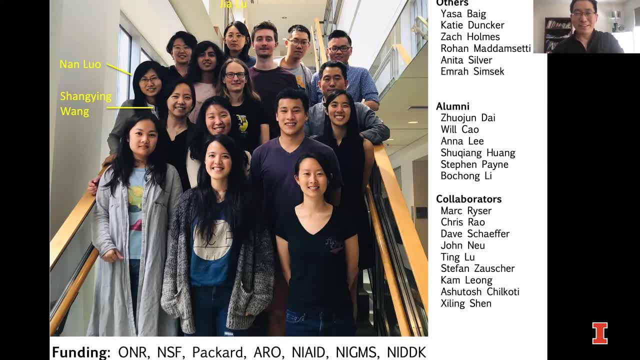 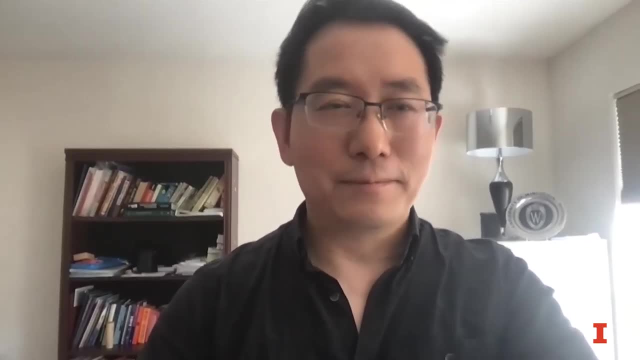 But explaining the pseudomonas branching pattern formation turns out to be a harder problem than we anticipated. So we actually spent several years just trying to understand the chassis a little bit more. I hope that clarifies your question. I have a question. This is Sergey Maslov. 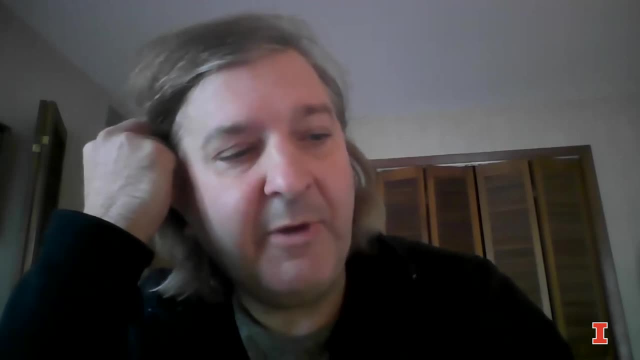 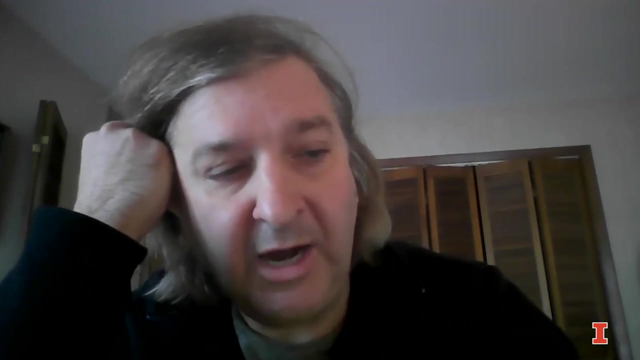 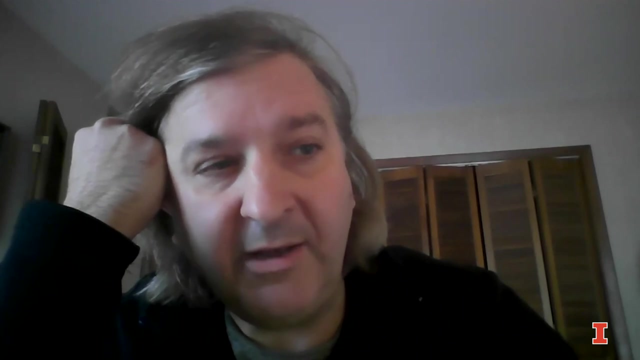 Thank you for a wonderful talk, Lingcheng. My question is about the part of the talk where you use neural networks to predict the outcome, the spatial profile of your simulations. So I can imagine that the parameter dependence is characterized by a fairly complex phase diagram. 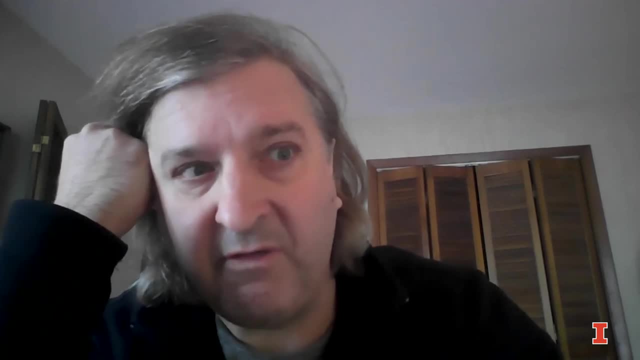 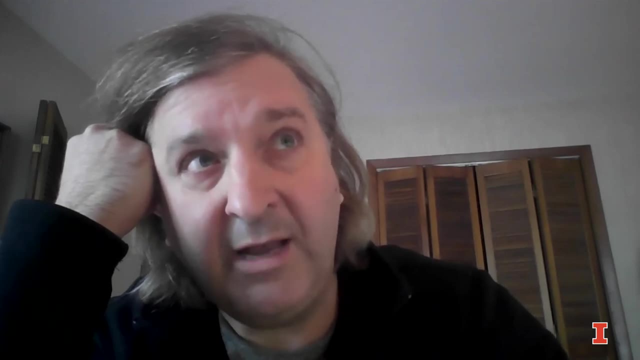 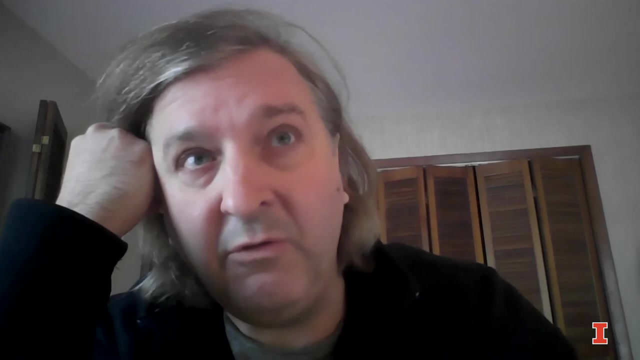 where you may have some discontinuous transitions. Is it possible that some of the cases where you had a large error between the predictions and the actual outcome are somewhere near those phase boundaries And, overall, whether you try to use your technique to actually just plot the phase diagram? 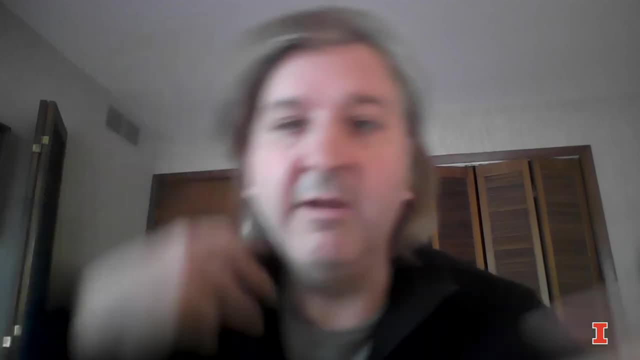 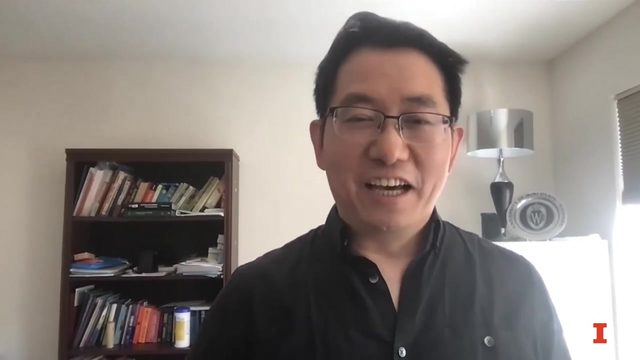 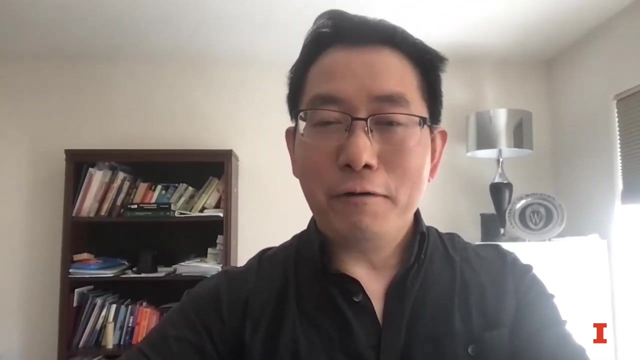 of your complex system of situations. That was a very, very insightful comment. I very much agree with your intuition. If you look at our discussion, that's precisely what we wrote: our speculation. We don't know for sure. The notion is that I suspect that's indeed the case. 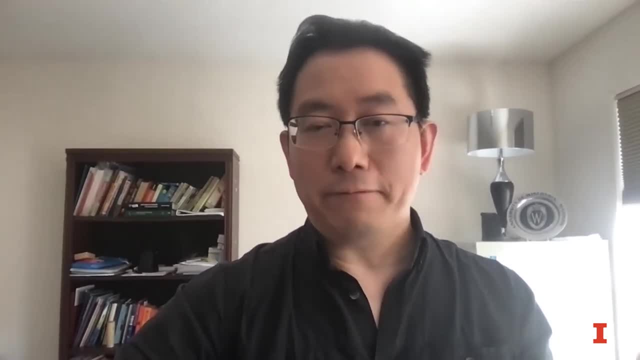 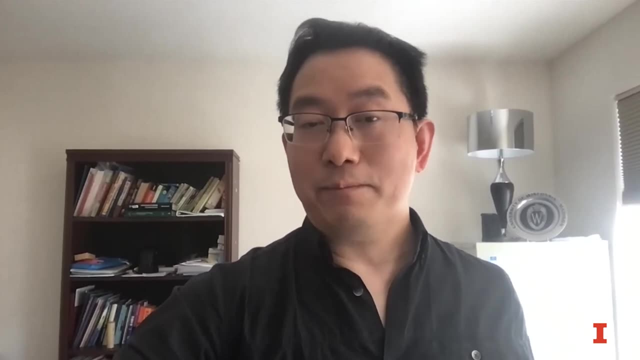 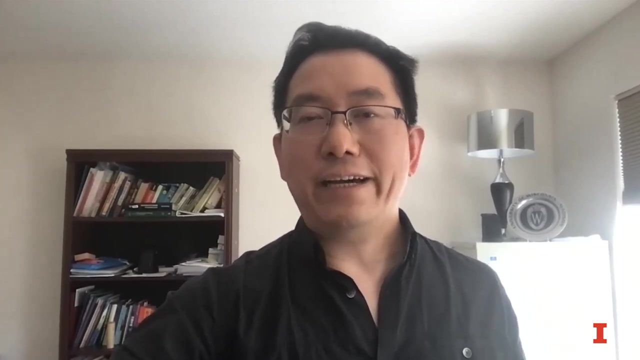 where, if you have system sensitivity being very, very high for whatever reason, if you have discontinuity, that's where the neural network can potentially fail In a way we have been thinking about. maybe we can use the failure of the neural network to map out. 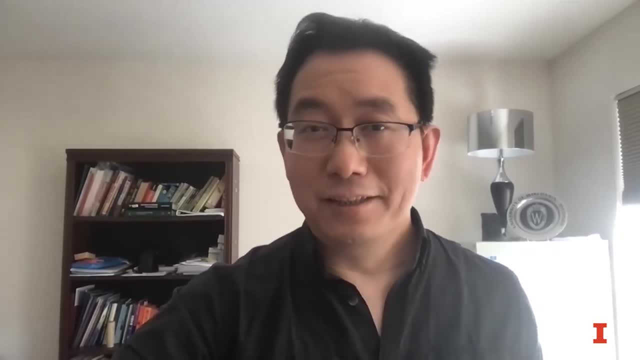 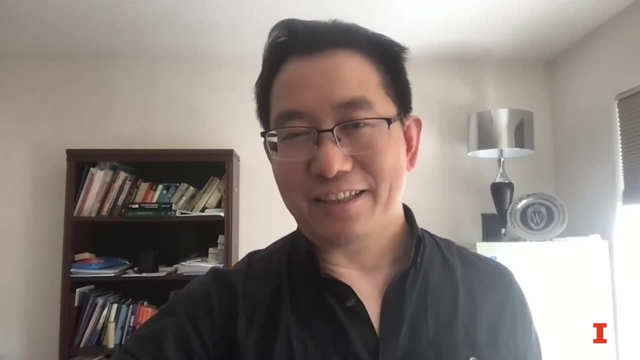 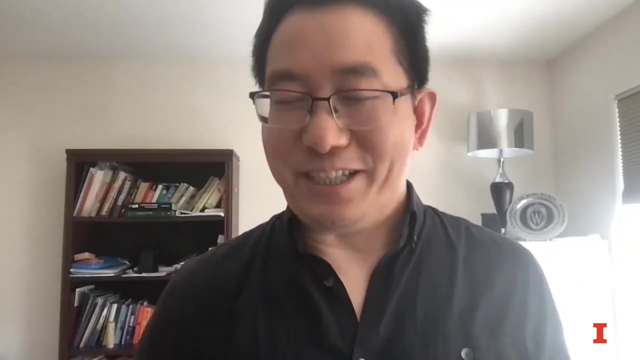 the sensitivity landscape of the dynamical systems. That's something we have been thinking about. We made some progress, but we don't have definitive conclusions yet. But that's a very insightful comment. Yeah, that's what we wrote in the paper actually. 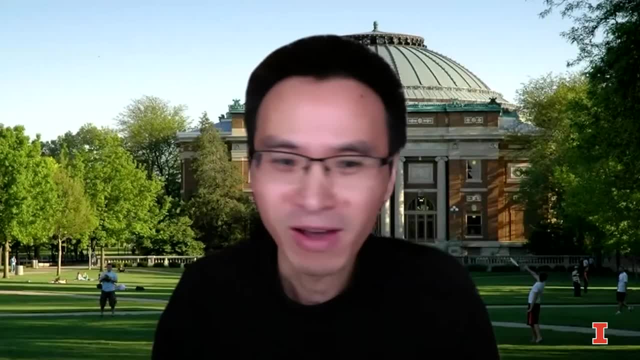 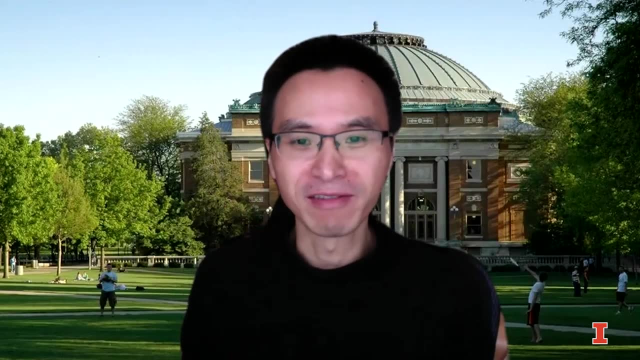 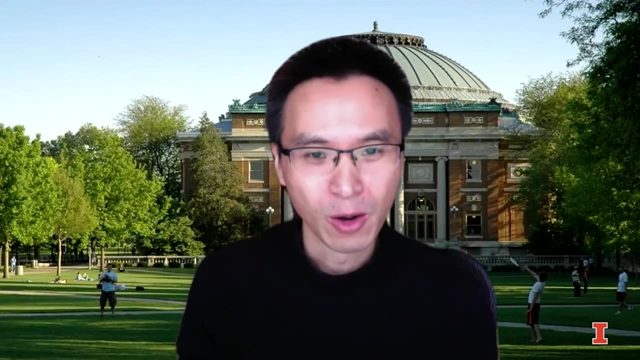 Thank you, Lingxuan. I have a question too, So it's a very general question. So, apparently, pattern-emerging from native living systems, such as monads, shown in your example, is often very robust and elegant, while those from synthetic strains. through the introduction of gene structure, are often noisy and fragile. So I assume that those synthetic strains may miss some key trait which may differentiate the behavior of engineered strains versus native strains. So I'm wondering: do you happen to have any insight about what we are missing? 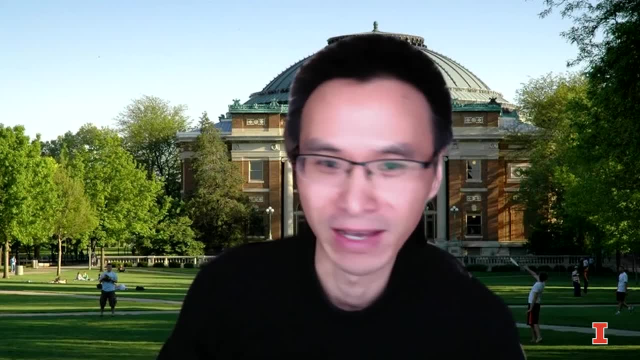 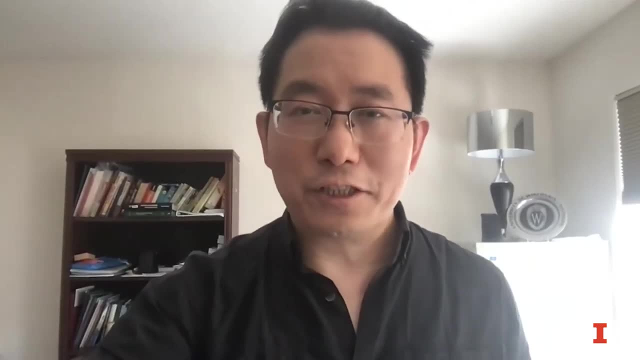 towards the creation of robust gene substrates that give rise to such a stable, self-assembled structure. Yeah, that's a fantastic question. This is something we're still learning. If I understand you correctly, you're saying that these pseudo-monads can form these branching patterns? 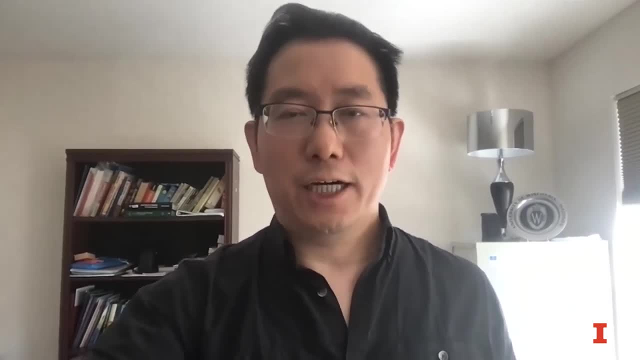 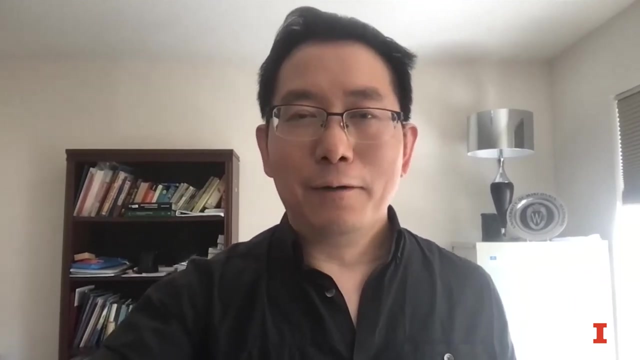 which are super reliable, reproducible. That's indeed the case. They are fragile in a different way. This is actually some result we're wrapping up a paper on. I can just mention very briefly. It turns out they're robust only if you always start from the liquid culture. 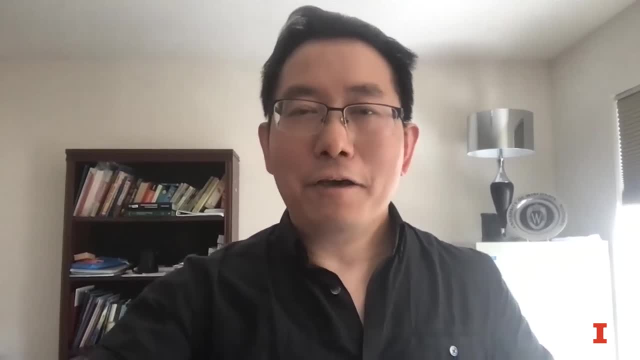 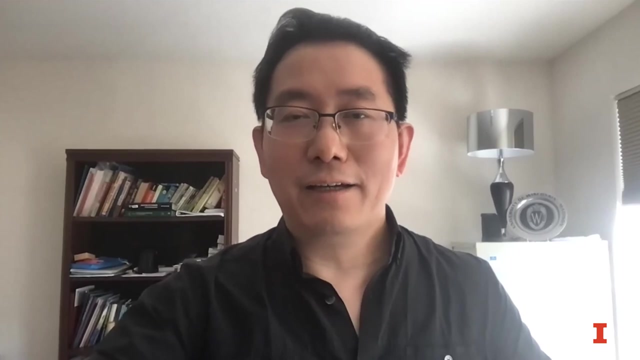 that's stored in the freezer right Now. if you propagate pseudo-monads on solid-phase that feature of programming- branching patterns can quickly change. It's very prone to cheaters, right, And that's one thing we are trying to better understand. So whether they're robust or fragile actually depends on the specific experimental protocols we're taking. We're not yet sure if these sort of patterns are more or less robust than some of the synthetic circuits we're building, But it's not necessarily a fair comparison. 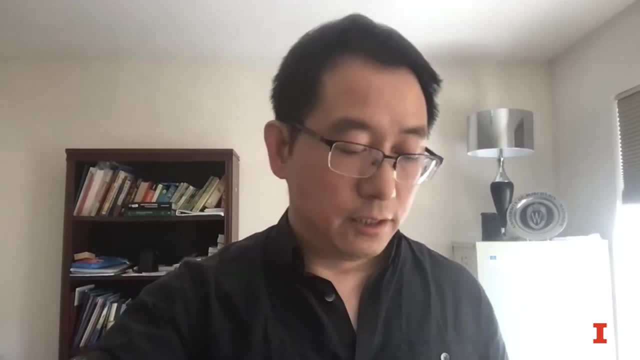 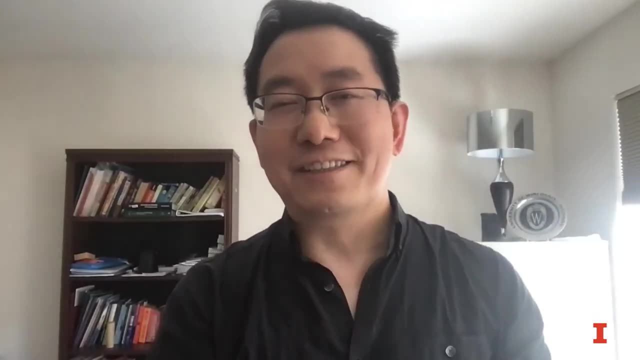 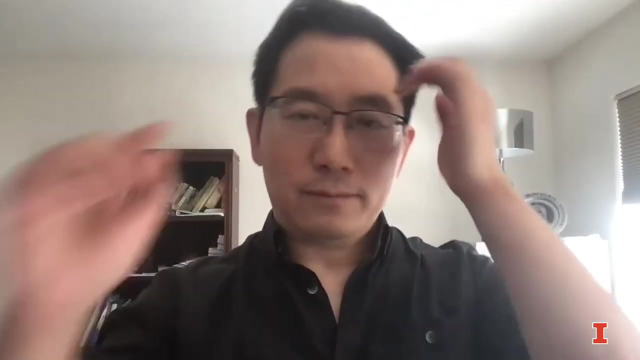 For instance, the ring pattern formation is quite robust, quite reproducible, But then it's also simpler. It's simpler, right, It's easier to reproduce that features, But the branching patterns it turns out to be quite dependent on how we grow the cells. 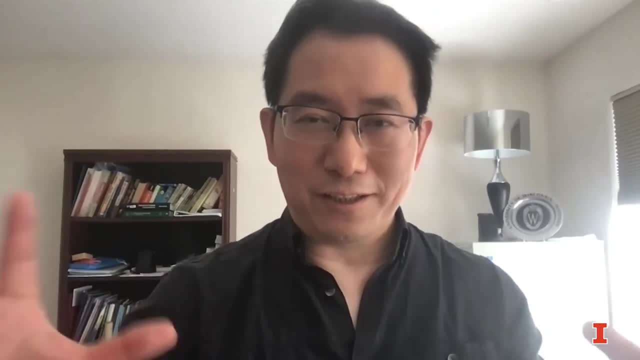 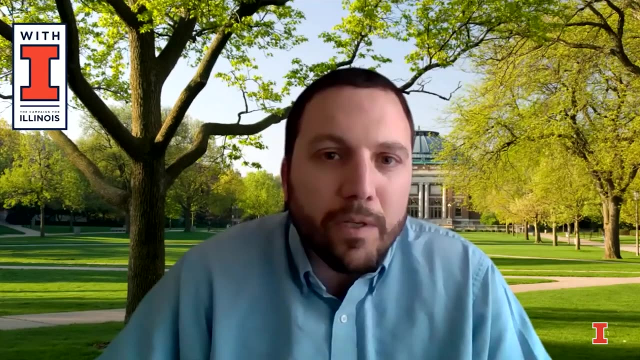 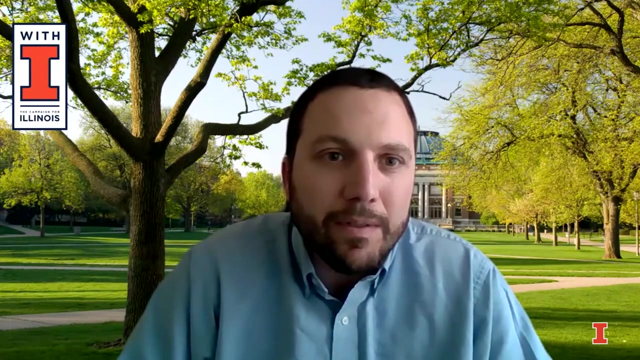 I actually don't know the answer to your question. In short, we're still learning. Reny Tong, have you tried, and what are some of the challenges in trying to grow 3D patterns? We tried a little bit, but we haven't tried hard enough. 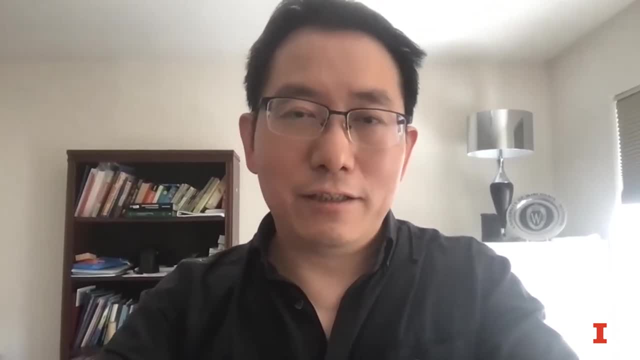 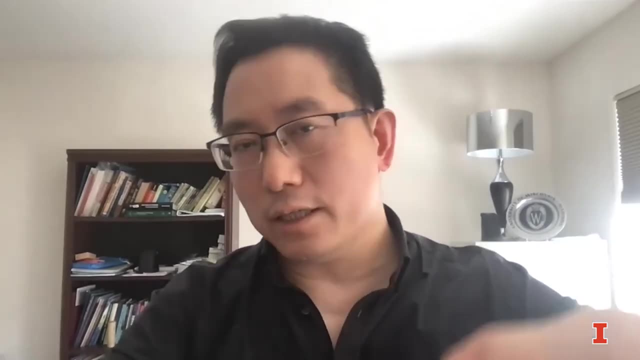 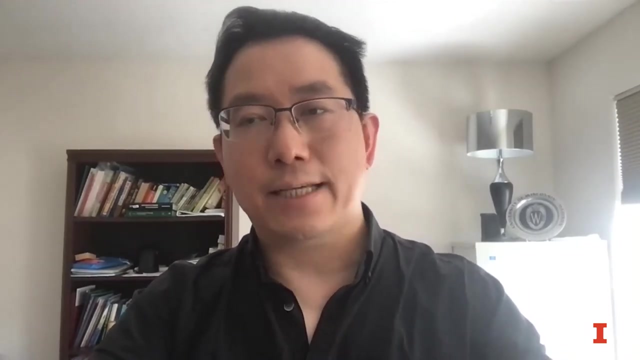 The little bit we tried is the example I mentioned in the literature biotech paper. We simply grow the cells on top of a membrane which allows us to control the nutrient flow and also make it easier for us to do downstream processing. And in that case,